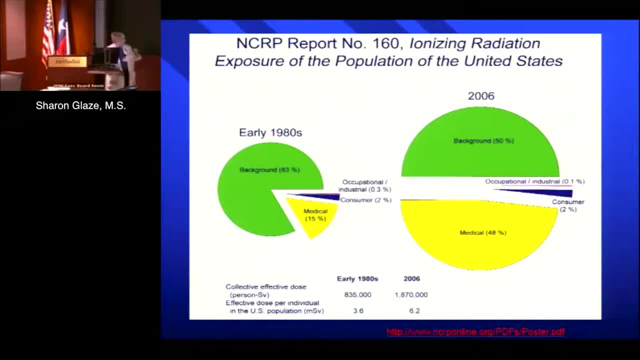 to happen. So in the early 80s the studies indicated that medical only comprised about 15% of the exposure to the general population in the United States and the rest came from background radiation in the earth and radon in the walls of the building materials in your home. So 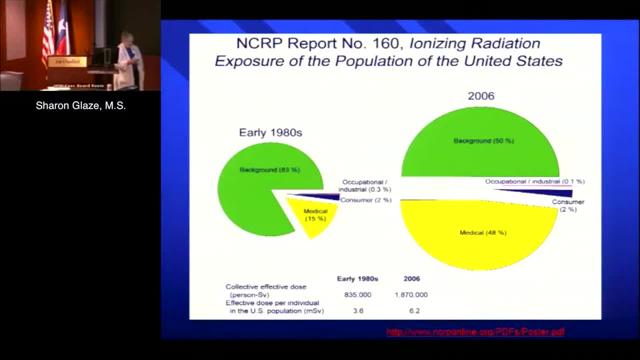 26 years later, this study showed that nearly half the exposure of the general population is from medical, And actually the effective dose per individual in the population has doubled, And so this certainly is a concern to those who don't know about radiation. So we're interested in radiation exposure to the population, And when we look how the breakdown 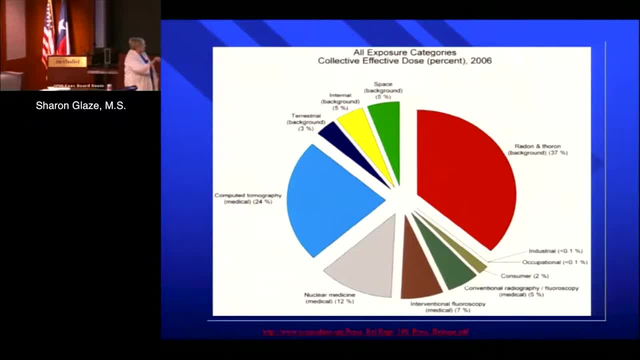 of this falls still. the largest part is from background radiation, but then the next largest chunk of the pie is from CT and then nuclear medicine, And because the doses for nuclear cardiology are higher, they are a large fraction of the population, So we're interested in radiation. 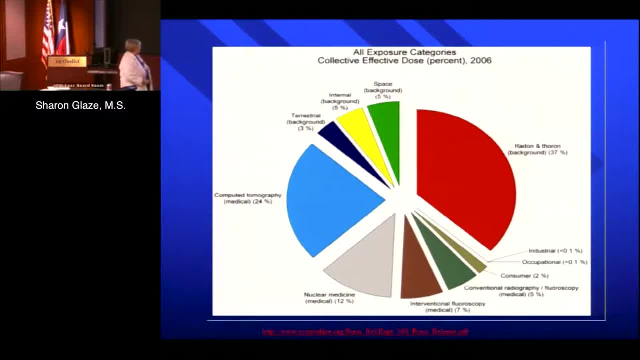 exposure to the population And when we look how the breakdown of this falls, still the largest part of this little piece of the pie And actually CT gets a bad rap because you know everybody going to the ER gets a CT nearly. And actually CT has saved a lot of lives and keeps a. 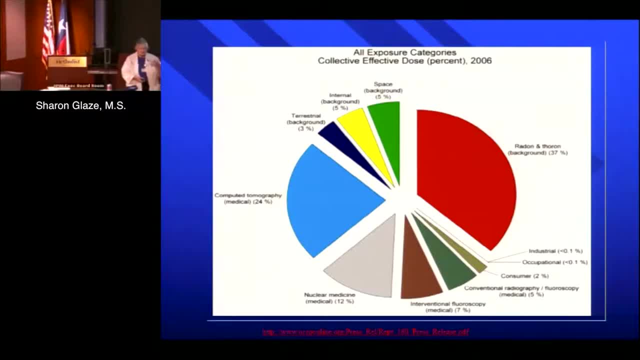 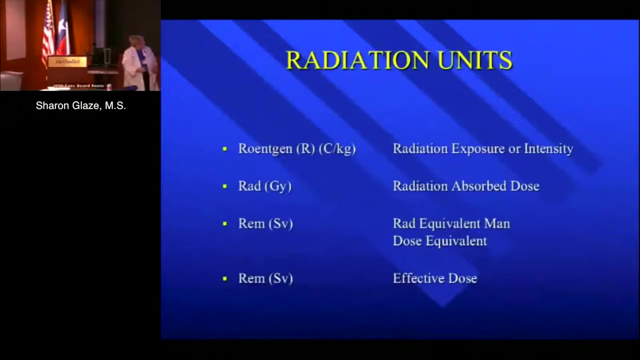 lot of people from having to have exploratory surgery, because that's what they did before we had CT, And so it's perhaps being misused in some situations, but it's a really important tool for us And we certainly can't do without it. So I haven't learned to work this gadget. 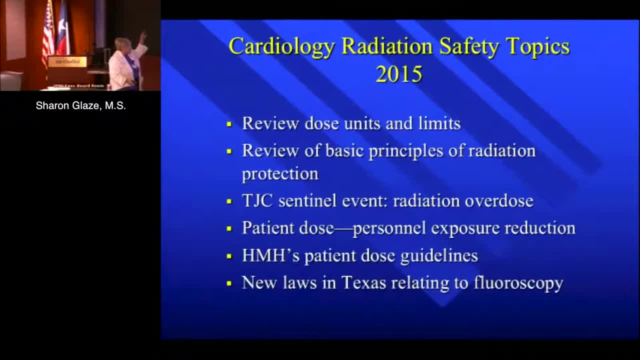 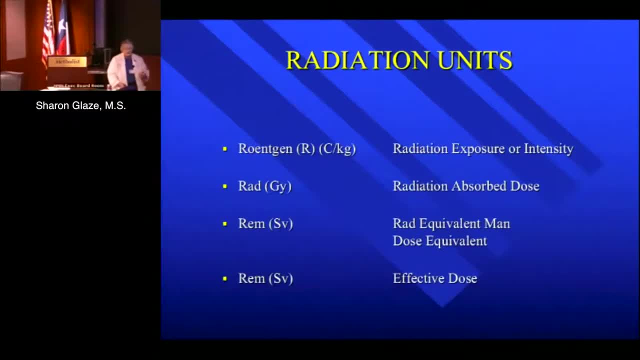 are. And then we're going to go over these subjects, some of the units and limits, because you have to have some small basic understanding of what these things are. And then we're going, because I'm the radiation safety officer here at Methodist, for all the x-ray equipment here and at Sugar Land. 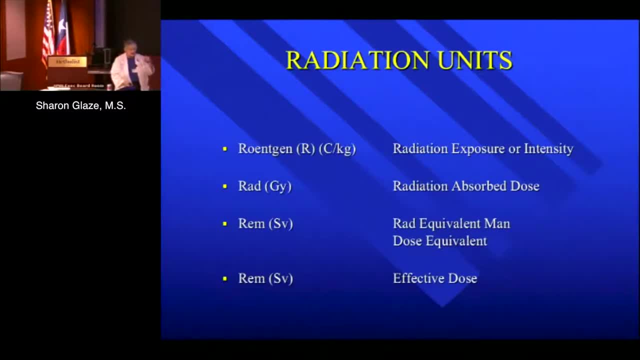 in Willowbrook and West, And also I take care of all the interventional equipment And so I guess through my career I've done about 1,000 cath labs. So I may look like your grandmother but I'm pretty into interventional fluoroscopy. 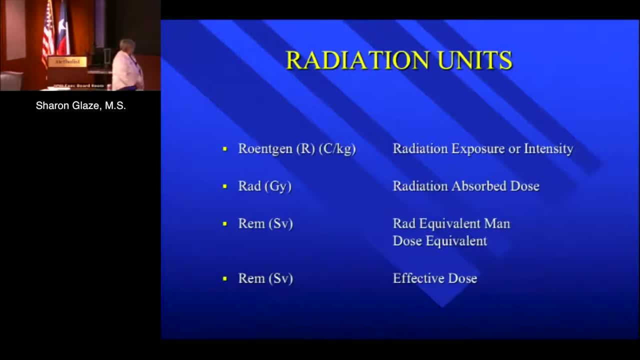 And so I'm kind of an unusual person. The second unit is the unit of absorbed dose, And so that would be the dose to some organ or to the skin in your case, if you've ever irradiated a patient. And the new SI unit is the gray. 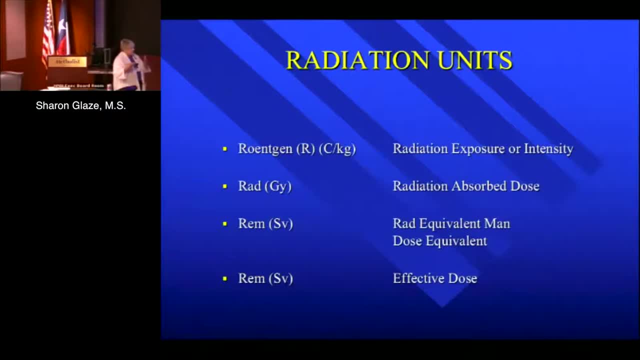 And so we're all trying. And where we grew up with liters and grams, we didn't grow up with rays, And so mentally I'm still trying to make the conversion. And the unit for your radiation exposure is the RIM or the Sievert. 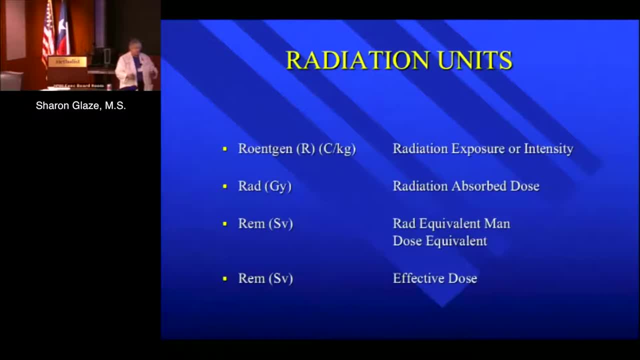 Here at Methodist and in most hospitals, we're still working with RIM and millirim. A new and important unit is the unit of absorbed dose And it's basically, if you irradiate my heart, what is the detriment to my whole body? 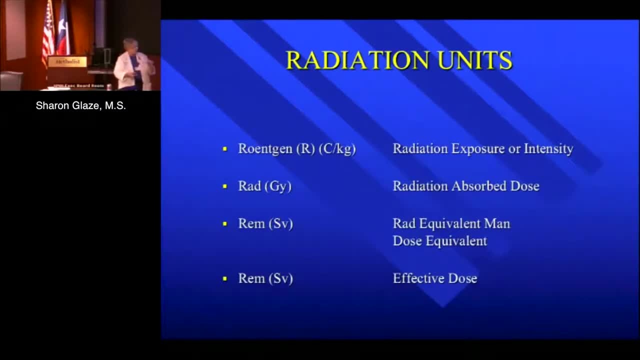 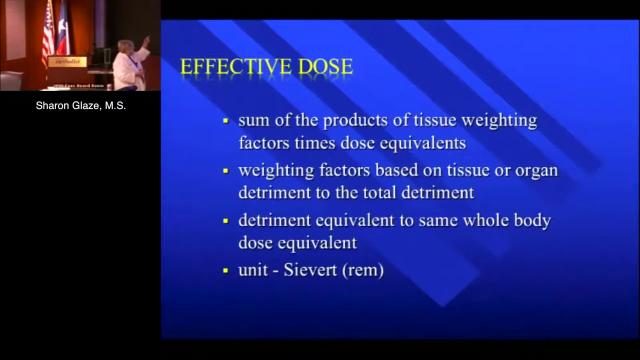 from having irradiated a small part of it, And so this is important in terms of risk, And if you do research, everything you do, you'll have to express what the effective dose was from that activity, And it basically sums the tissue weighting factors. 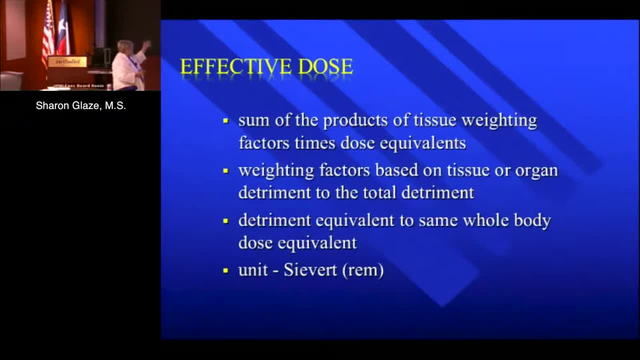 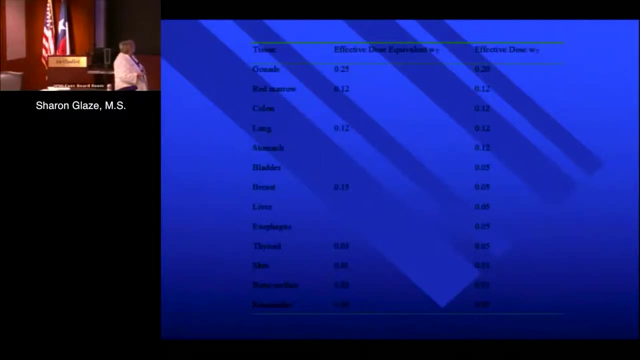 and helps determine the detriment equivalent from the same whole body exposure, as I said, And the unit is the Sievert. And here's an example of some of the weighting factors. If you ever need them, you can easily get them over the internet. 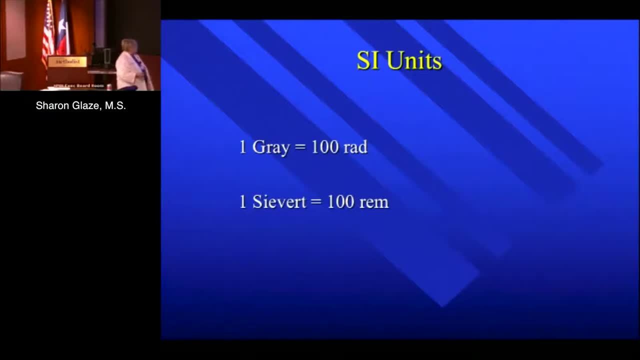 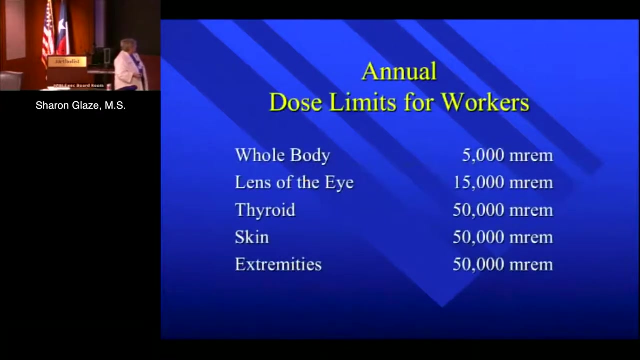 And so this is the SI unit. This is the difference. It's a factor of 100 difference between a gray and a red, And so my brain's working on that. In terms of personnel protection, every year we provide you monitors. They're supposed to be worn at your collar. 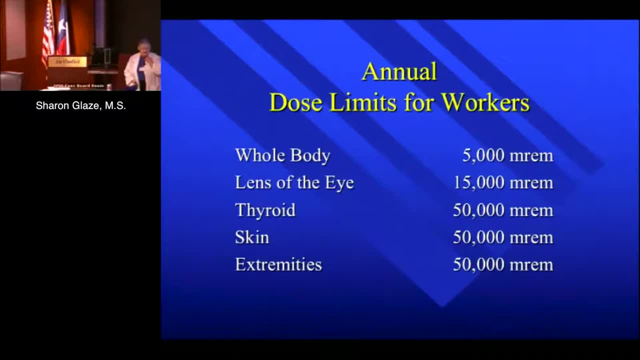 which stabs you right in the neck while you're trying to cath. But they provide you monitors. They put them at the collar because this is the unprotected part of your body, your head, And it also is used to calculate the dose to the lens of your eye. 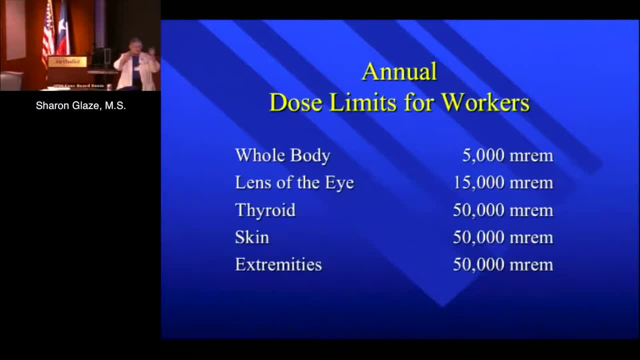 because heads are about the same size and they apply a correction factor and estimate the dose to the lens of your eye. So the limits have not changed for the whole body in the 40 years I've been doing this, And so it's 5,000 milligrams. 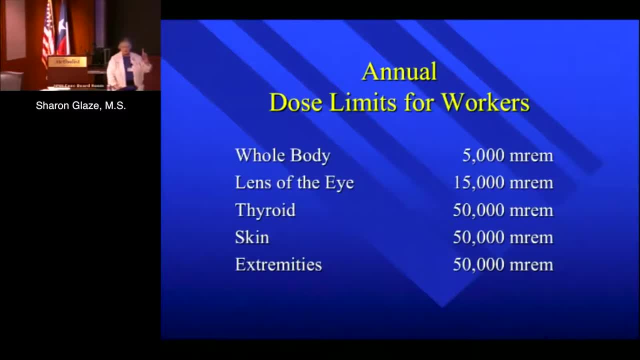 Who are the only people in the hospital that approach this value, Cardiologists. So you need to wear your badge so you can learn what you're getting and monitor how you change your behaviors, how you can reduce your dose. The lens of the eye dose has changed. 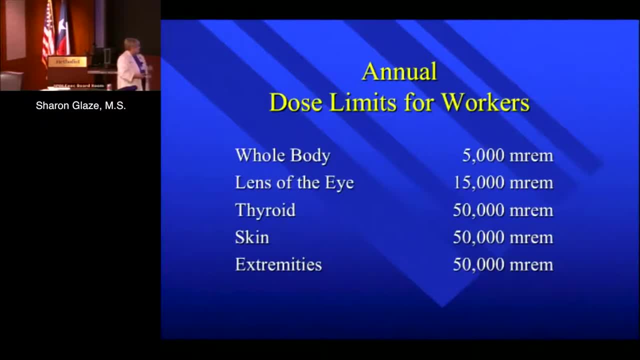 They decided the lens of the eye was going to be the eye. They decided the lens was less radiosensitive than they used to think it was and it's now 15,000 milligram or 15 rem. And then the thyroid, the skin and the extremity limits are 50 rem. 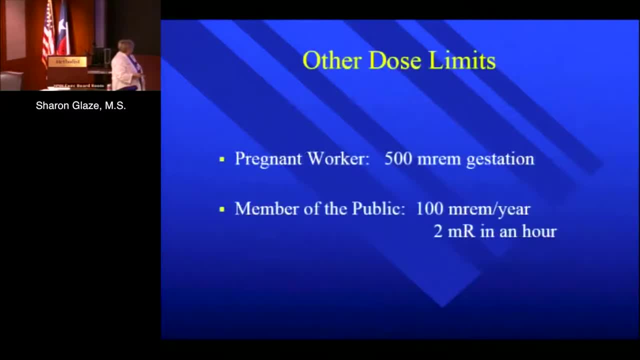 per year, or 50,000 milligram. There are other dose limits. Pregnant workers are less likely to get the vaccine. They are limited to 500 milligram during the gestation because the fetus isn't a radiation worker, And so they didn't sign on for this. 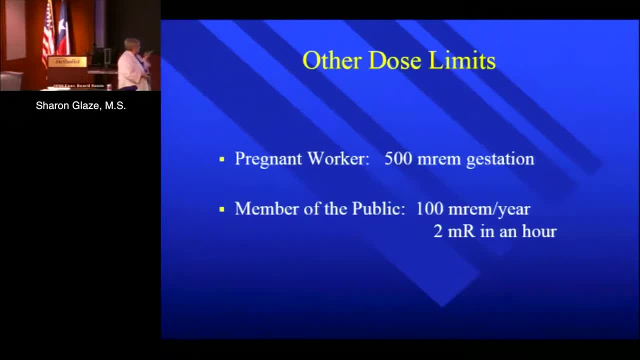 And so we have to monitor them very carefully. And then members of the public: we have to limit their exposure to 100 milligram per year, or 2 milligram in an hour, And sometimes this can be a challenge. One example of that is pet facilities. 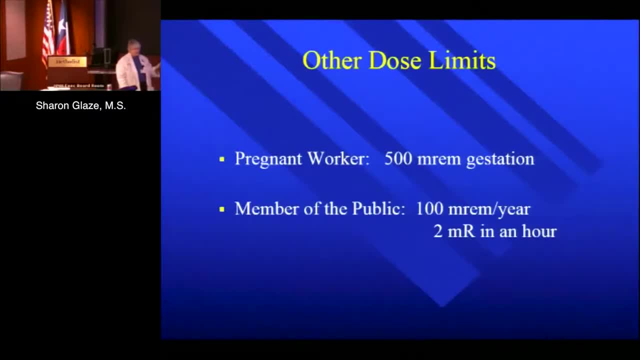 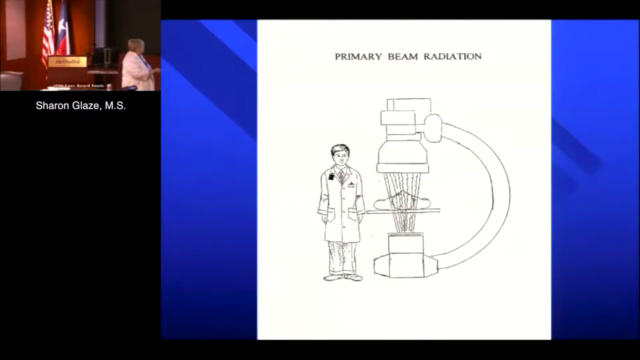 That can be a challenge, because at 511 KEV the exposure rates can be high and it takes a fair amount of shielding. So where does your radiation exposure come from? Well, when we use the primary beam pointer, it doesn't work on this blackboard very well. 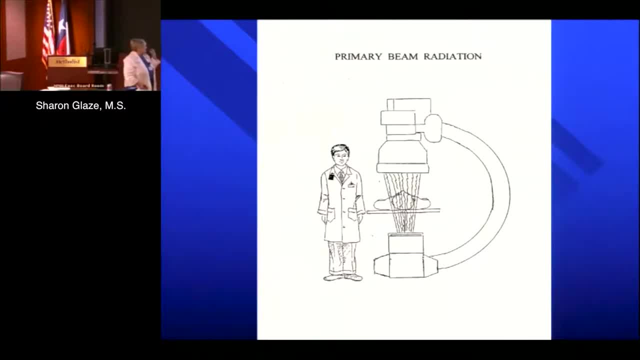 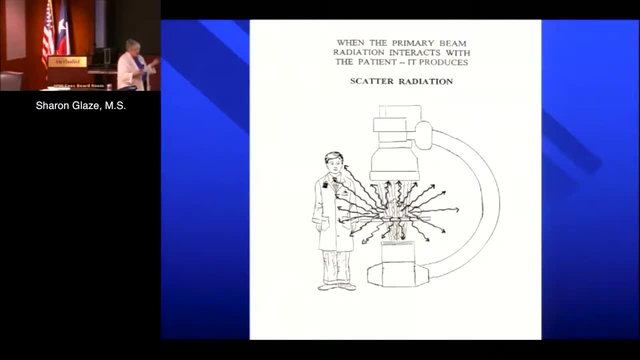 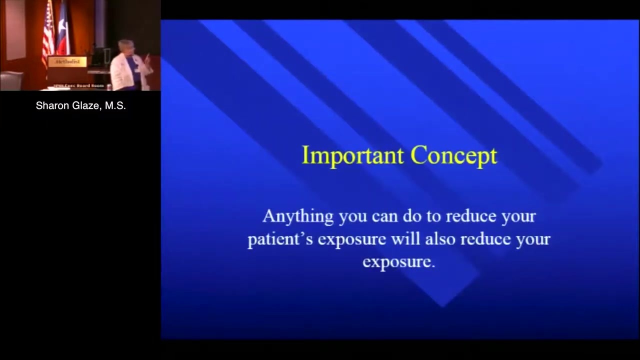 When we use the primary beam to create the image, it interacts with the patient and produces scattered radiation that is of a much lower level, but nevertheless it's proportional to the entrance exposure to the patient. So here's an important concept: Anything you can do to reduce your patient's exposure. 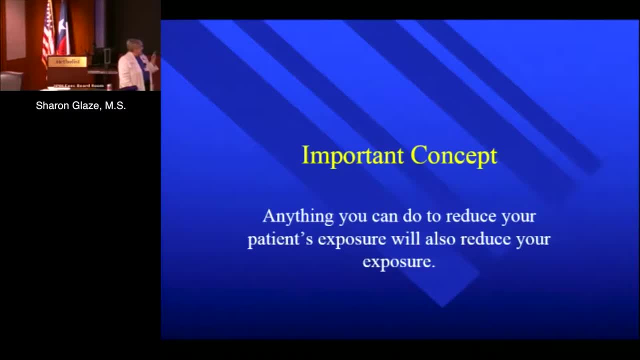 it's also going to reduce your exposure. So it's important that we use the lowest dose equipment we can for both of you- your patient and you- and do other things we can do to reduce the exposure rates. So the basic principles of radiation protection are the same, whether we're dealing 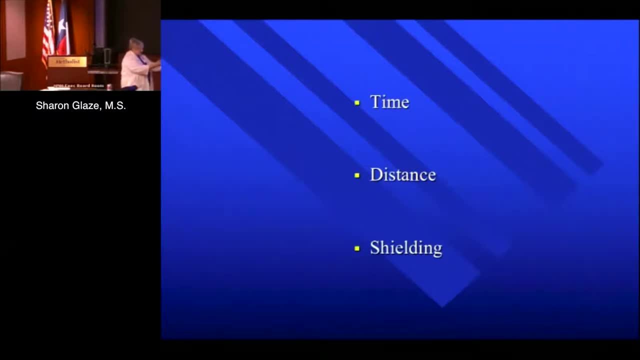 with something that's going to be a high dose or a low dose. So the basic principles of radiation protection are the same whether we're dealing with something that's going to be a high dose or a low dose. So the basic principles of radiation protection are the same whether we're dealing with something. 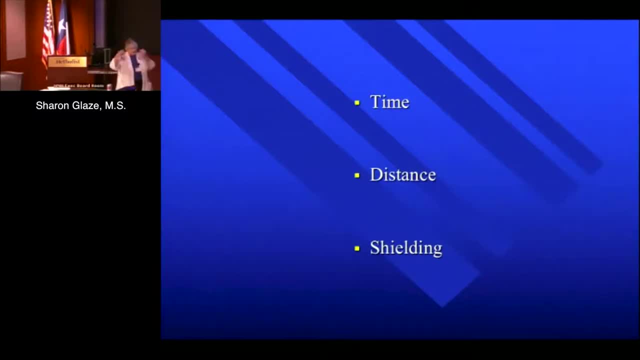 that's going to be a high dose or a low dose. So if you have a patient who's been attacked with a dirty bomb or a cath lab or a nuclear reactor, it's time, distance shielding, And so, in terms of time, there's a little more of a sermon for you. 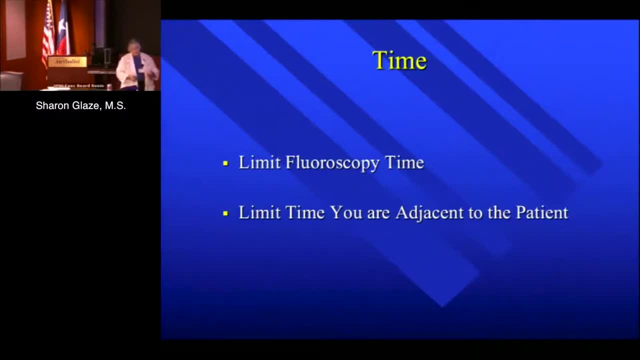 because you control the fluoroscopic time. So it's important to try to learn to limit your fluoro time. I catch myself all the time here you're managing the fluoroscopic time. We'll do it again in a minute. So the basic principles of radiation protection are to reduce your exposure to oxygen. 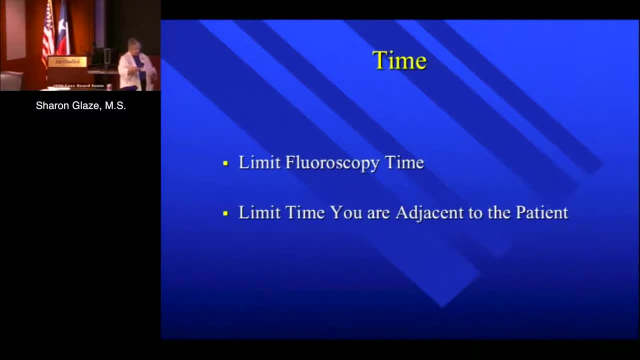 the medical aspect of the patient. you're trying to do a tedious, delicate little thing and think about what's coming next, catch myself all the time with my foot still on the pedal when I'm not doing anything, and so you have to train yourself, starting in the beginning, to watch what you're doing in terms of how. 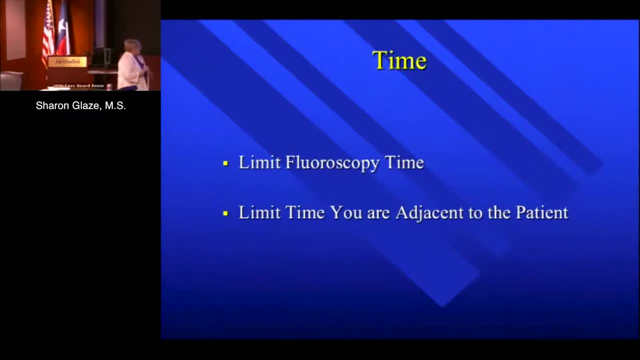 long your foots on the pedal and so maybe you know- just hearing me say this will help you think about that during your career. it's important that you limit the time you're adjacent to the patient, because that's your source of exposure, not that evil x-ray machine. it's the patient that's exposing you. 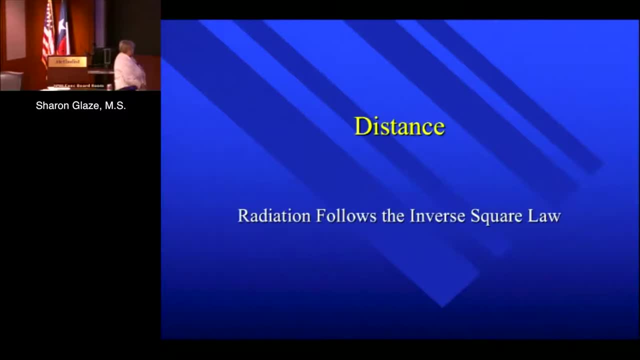 because of the scatter radiation there producing, and so radiation follows the inverse square law. so this is the patient, and I'm a bit from the patient, if I can step back another foot. I've doubled my distance and my exposure rates, down to a fourth of what it was. 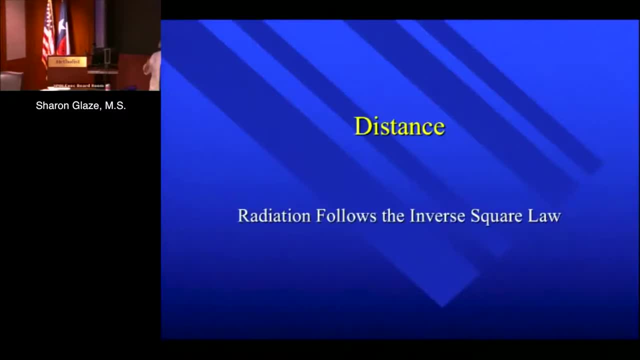 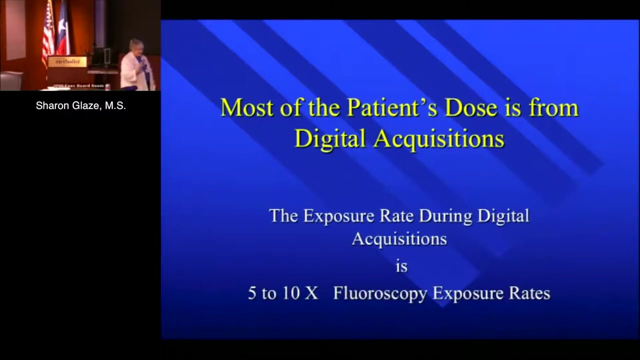 when I was standing next to the patient. so one little foot makes a whole big difference in cutting your exposure rate. so obviously. but I stuck this slide in so everybody thinks I'm doing a lot of flora. that's the biggest problem here in the room, but actually the biggest. 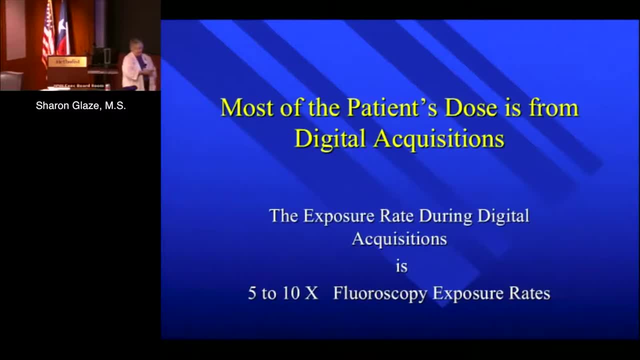 problem is the digital acquisitions, because the x-ray unit runs at five to ten times the exposure rate during a digital acquisition that it does during fluoroscopy. so it's kind of important- I know you're trying to hold the catheter still and whatever you're doing- but if you can somehow step back during your 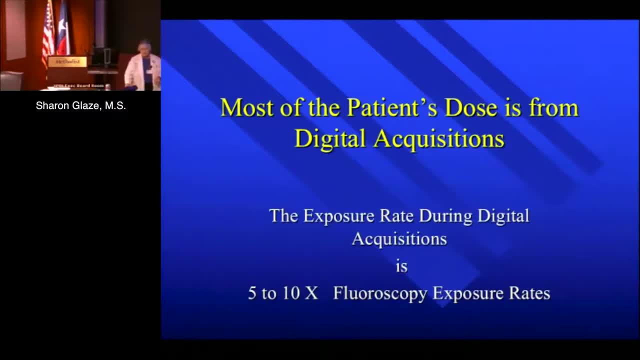 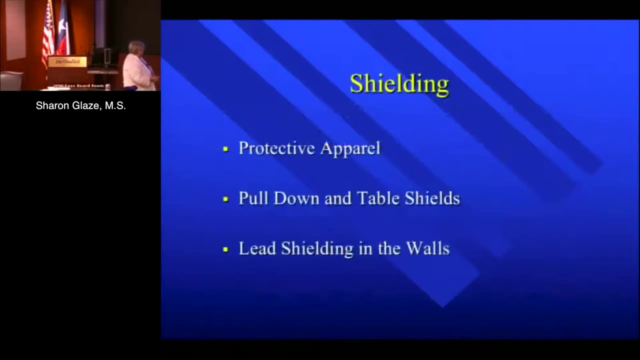 digital runs. it'll really cut your exposure rates down a lot, because if you don't, you're not going to be able to do it because they run really seriously five to ten times higher during digital runs. and then we provide protective apparel to you and you need to learn to use your table shields. so here's an. 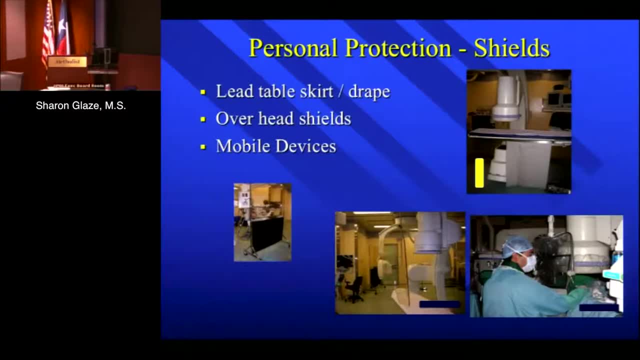 example of this one. it's nice with the pull-down shield when you can use it, but some facilities have a lid drape and that helps keep the scatter from coming under the shield at you. unfortunately, ours don't. but you have to remember it's not just hanging up here in front of your face, you need it between you and 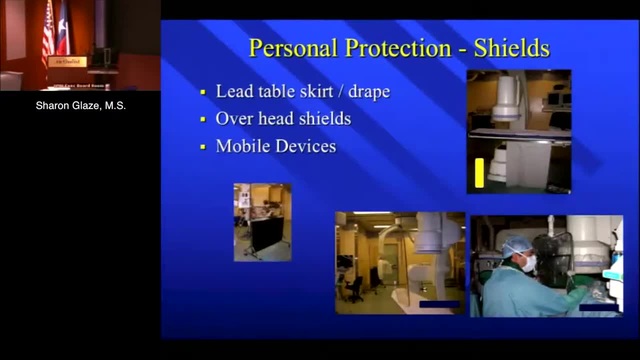 the patient to have it do any good, and this little gadget is really important. these table shields: I hate those things. when I go to test the room, the first thing I do is try to move them out of the way. but you guys can't do that. they did a study of cardiologists and 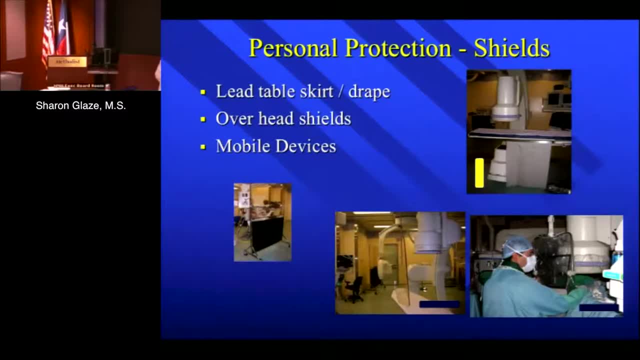 most of them had no hair on their legs, but the time they were like I don't know how old- 50 years old- and they had epilated their hair on all their legs, and that's where they had their hair on their legs start, that's when they started putting these table shells in. so if we had women 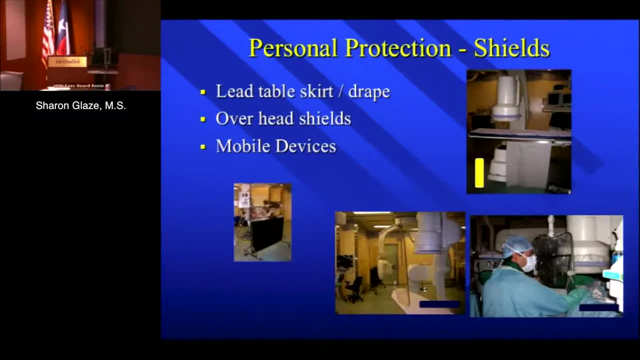 here I could say: well, you won't need laser hair removal if you don't use your leg shield. so I'm really serious, you need to learn how to use these, because the problem is the x-ray tubes under the table and the primary scatter hits the table and the patient and bounces right back at you. so those leg shields. 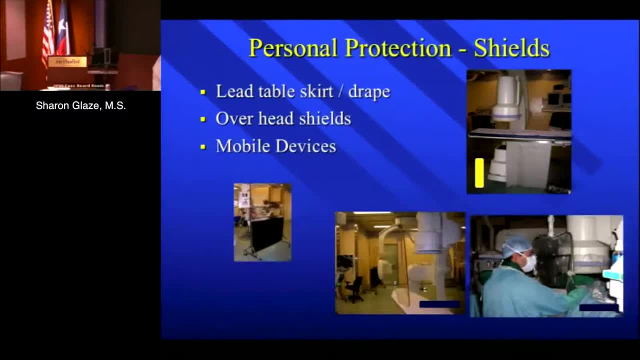 they're so annoying are really important. so try to keep learning to use those and to work with them. fortunately, you work from the groin, so you're a little bit further back than I am when I'm filling with these machines. yes, are there certain views in which there is more scatter? so I hear that PA, and there's. 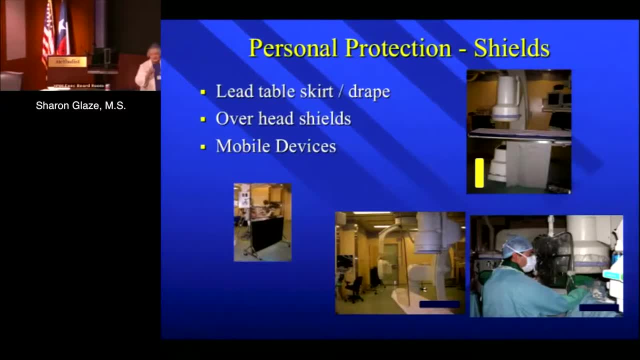 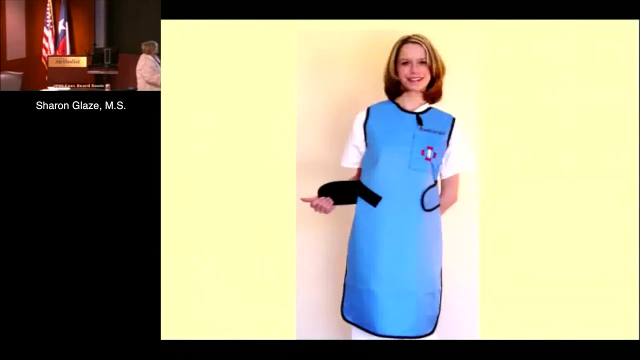 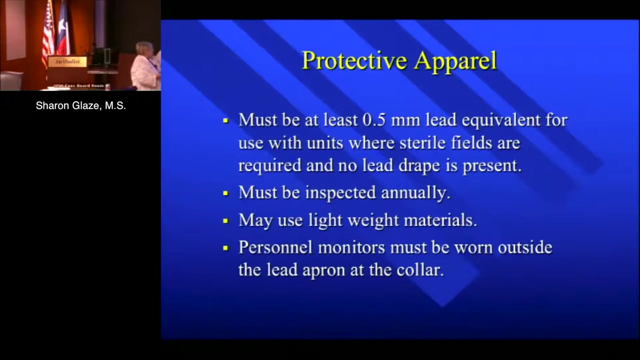 less scatter when the when the tube is straight up and down. I'm gonna have a little slide to show you. it may be coming up short, but okay. so in the cath lab we try to. well, we do have only half millimeter lead equivalent material actually in the. 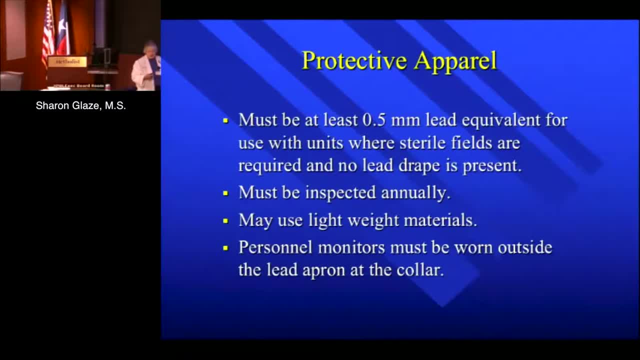 whole house. we have only half millimeter. they make thinner lead equivalent materials that we try to provide you the best. however, we will also provide light white materials which are kind of. they're very proprietary, they're they're little recipes and we'll try to get them to sort of create a 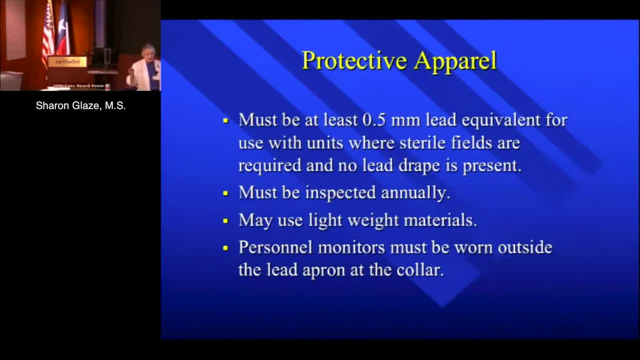 saw their own made of high seam materials like copper and bismuth and zinc and different things, to be lighter weight than actual lead, and they often have a lead mix in as well, And so we provide those to you and need to make you aware of a couple of things which 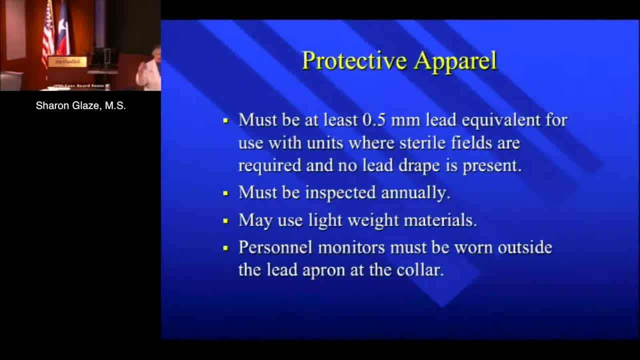 is, the backs are usually a quarter millimeter and if you have a wraparound thing it's usually quarter millimeter on each side. So if it doesn't fit you properly and doesn't wrap around correctly, you're getting like a strip of half millimeter and then two sides of quarter millimeters. 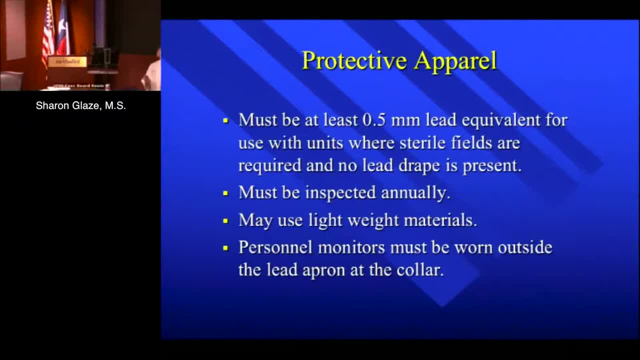 So you really need to have an apron. They fit you correctly so that you've got the whole wraparound lead equivalency And you know you need to. we're trying to make you the radiation safety people in the room And if you see nurses- because I see it a lot, a lot of large busted nurses, the thing. 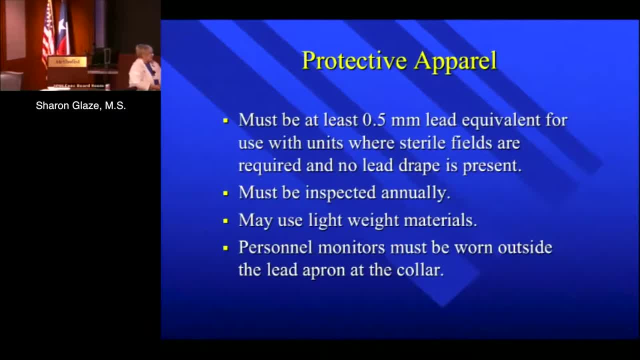 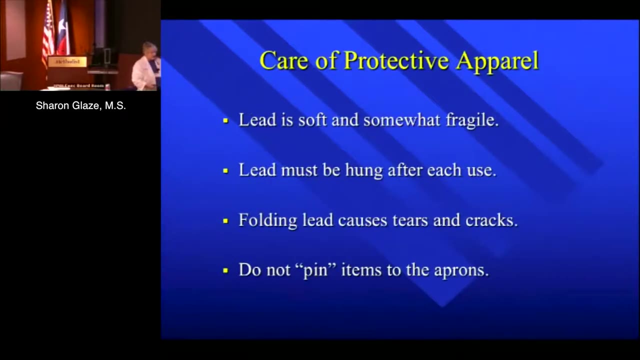 doesn't quite fit them correctly, And so when you have your own practice, you need to make sure that Okay, You know your people are outfitting correctly Leads very soft and tears easily. It needs to be hung and on proper racks. 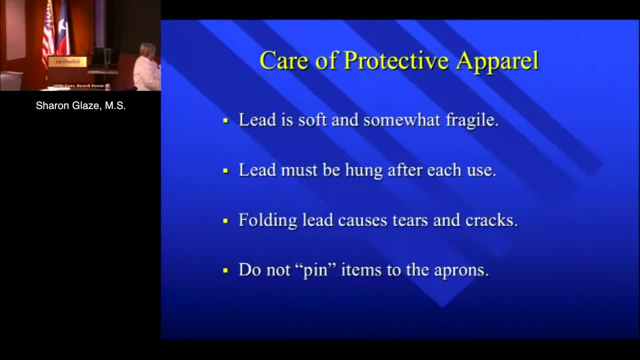 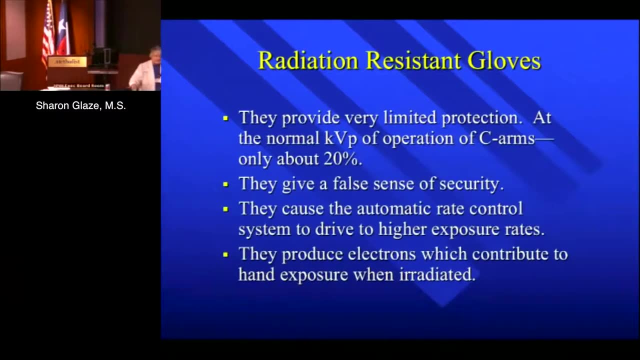 If you don't take care of it, it won't take care of you. And let's see, what else can we talk about? There are some things called radiation resistant surgical gloves. Have you ever seen them? Nope, The pain medicine. people are really into them. 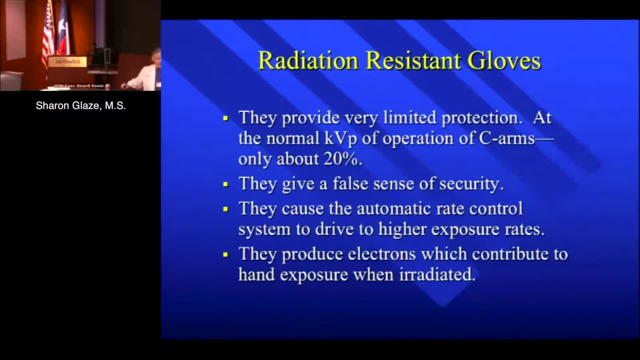 Somebody teaches them they ought to be using them, But they actually are only 20% protective. That's why they can't be called protective. They're called resistant And they're really a problem because these x-ray systems have sophisticated automatic brightness systems on them. 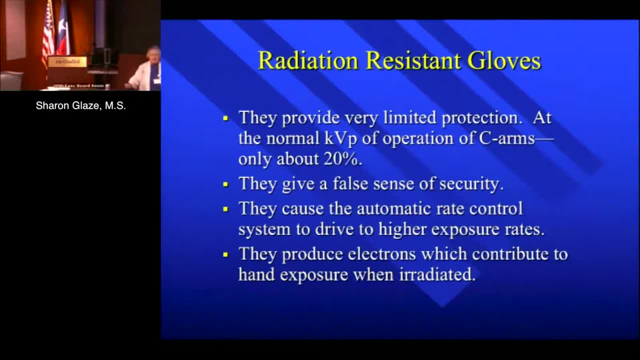 So when you move from the chest to the thick abdomen, they adjust the rate so you can see what you're doing. And when they see these low protective gloves or radiation resistant gloves, they shoot the dust rate up really high And they're only protecting 20%. 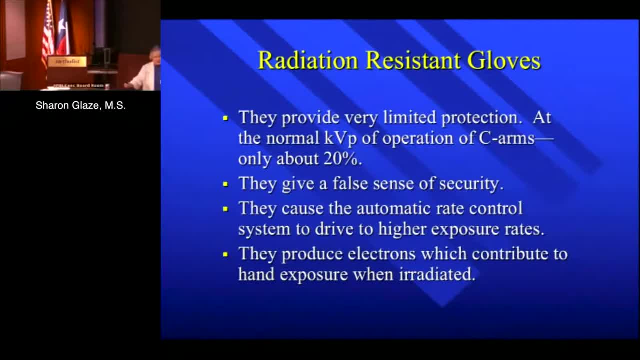 So your hands are really getting irradiated more, So don't let people talk you in. Just try those gloves. They're not a good idea. Okay, Here's the answer to your question. There isn't much you can do about it. 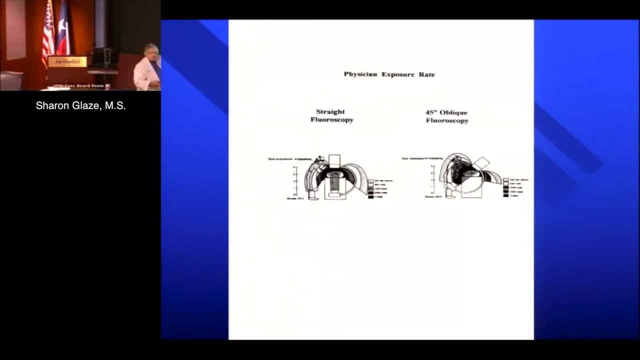 But when the unit's straight up and down, if you see this darker shading, it's kind of down in your apron and in your chest in a protected area. But when you have to angle the unit then it comes more up toward your face. 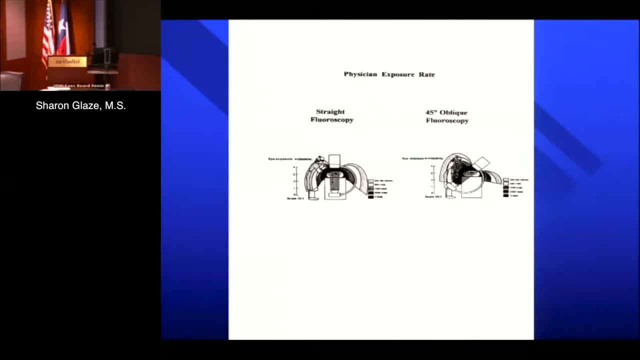 Okay, But if you're using that pull-down face shield, then that helps protect you from that. But yes, the scatter rates are higher when it's angled. So another question, sorry: Is the patient exposure also higher? Because, you know, I recently was told, you know, this patient had one long procedure. 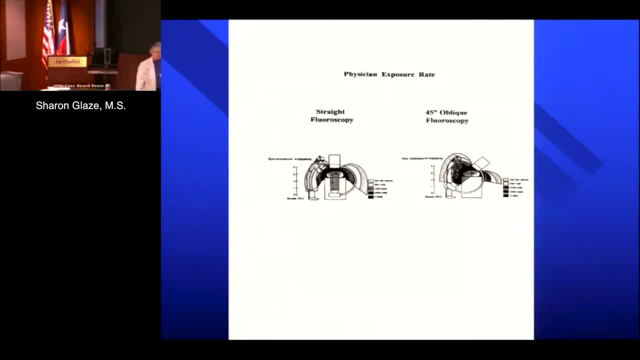 where they used a lot of angulated shots and the radiation dose at the end of the case that's measured was a lot higher. And the explanation that was given to me was, well, that because of the fact that they used a lot of angulated shots, the patient dose was higher. 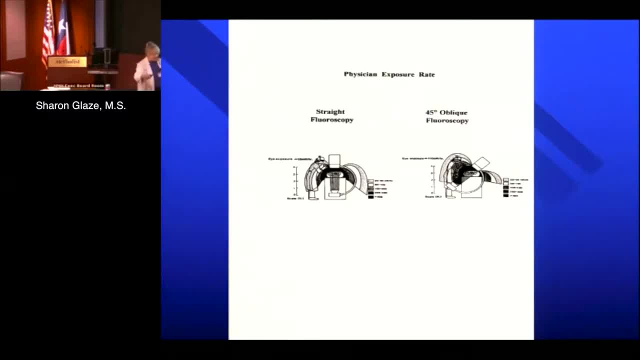 Now does that? So I suppose. so If you're using some big angle and it's going through a thick tissue amount, then it's going to have to run the radio to penetrate that. So So does the machine. Since I don't go to the procedures, I don't see these, but it's conceivable that what? 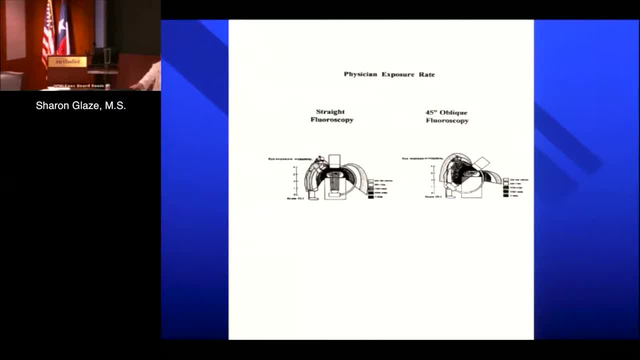 you're saying is true. So I'm not sure if this is true, I'm not sure if this is a question that you can answer, But the machines are they programmed to run in a way where, if you know, if it's a heavy? 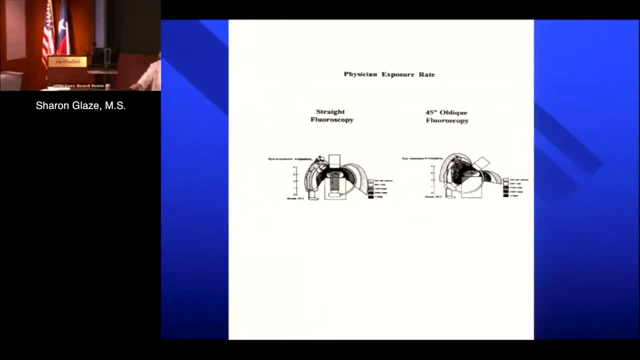 patient, for example, or it's an angulated shot and there's less reaching the eye-eye, does the output automatically increase to compensate? Yes, It does They. I don't know exactly in the modern equipment how they do it, but in the older days they. 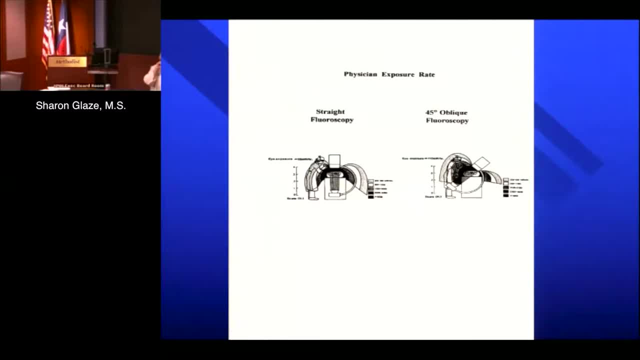 used to have like photomultiplier. Like photomultipliers that sensed how much light they were getting and they raised the rate to adjust for it. We have different methods with the digital equipment But the answer is yes, It definitely adjusts the rate. 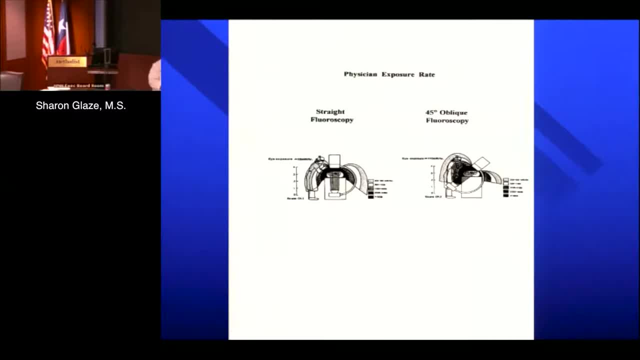 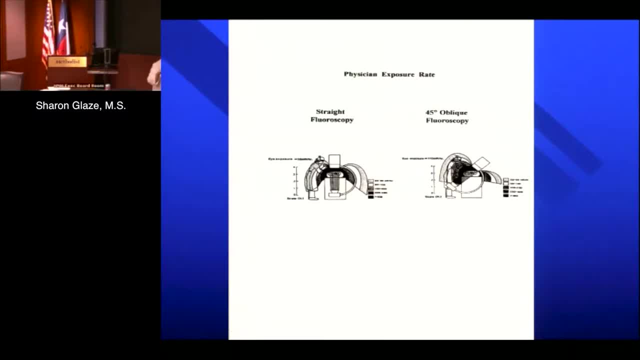 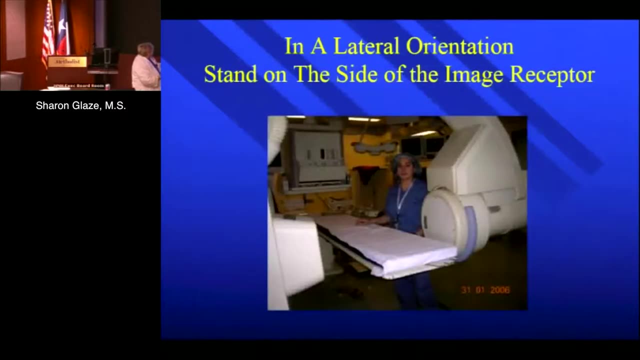 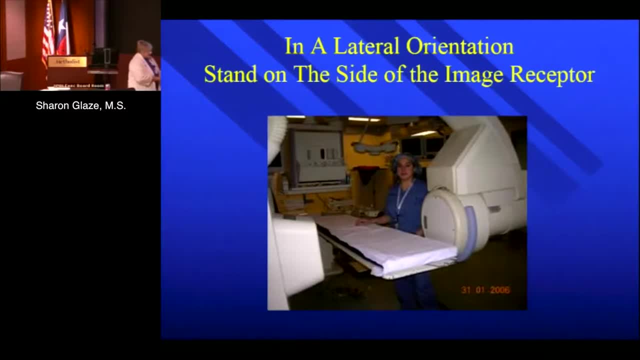 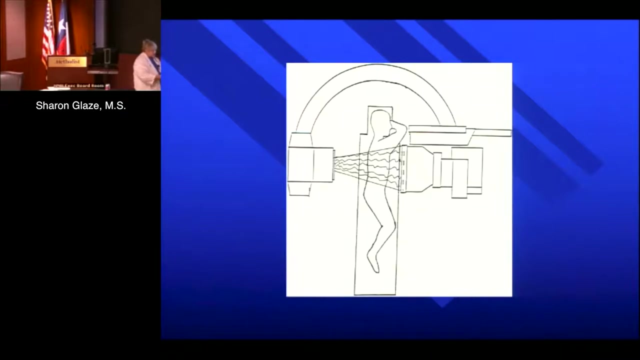 But in the lateral orientation. in the cath lab you usually do them at 45 degrees under the table, so this is more like haploidal boulder neuro. But you should stand on the side of the image receptor Why? Well, the reason is it's kind of like the tube under the table with your legs thing. 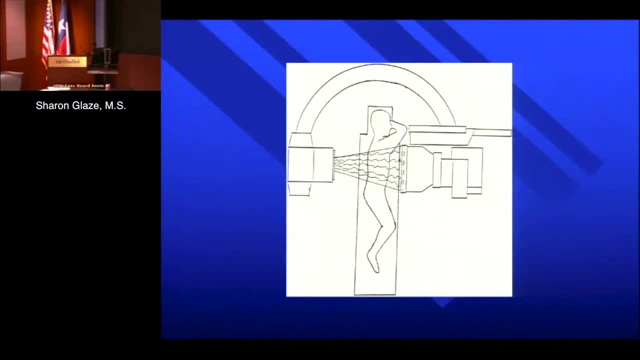 We check very carefully to make sure the beam's collimated correctly. Now if the beam weren't collimated correctly and you were getting primary beams, then that wouldn't be good. How can you control that? You can have the tech bring the shutters in so you can see them on the screen. 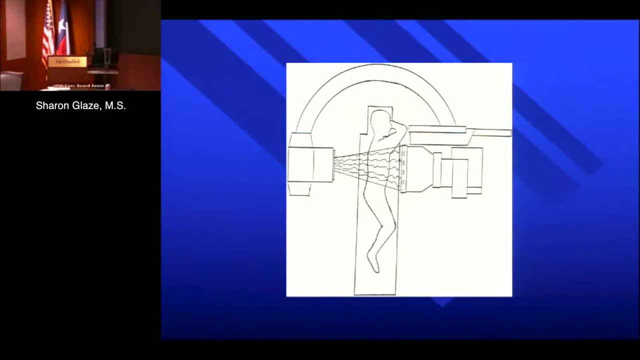 And if you see these little square shutters you'll know there's never any primary beam going outside the detector, And here on the X-ray tube side, you're getting the primary scatter back in your face. So it's better to be on the other side but to collimate in, so that you know that some physicists like me 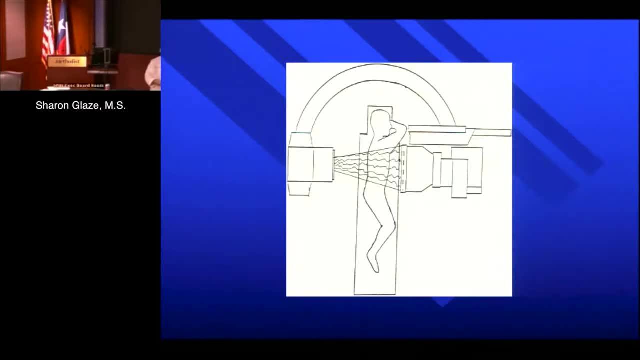 didn't make it. They didn't make a mistake and that the shutters are really there. So a lot of them are irises and you can have it brought in. So to me, this is the kind of information you guys need to know, and so I hope it's helpful. 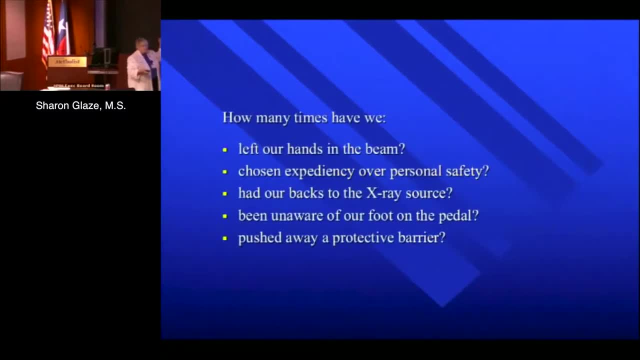 Positioners, We don't make any. How many times did you lift your hands in the beam because you didn't want something to move? Chosen expediency Over personal safety? Had your backs to the X-ray source, Been unaware of your foot on the pedal? 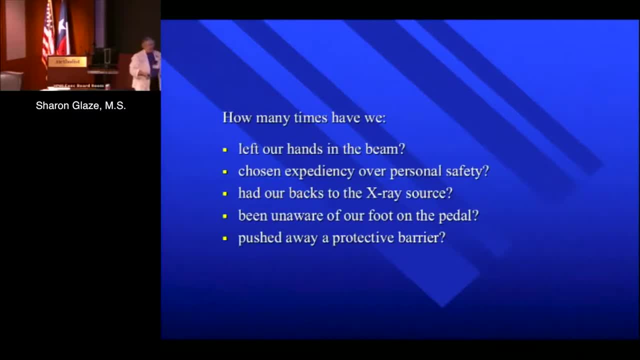 That's my big sin- And pushed away a protective barrier. So you know you need to think about what you're doing because this is your whole life. I do like to see you wear wrap-around aprons- So good examples. We had one surgeon out in Sugar Land. 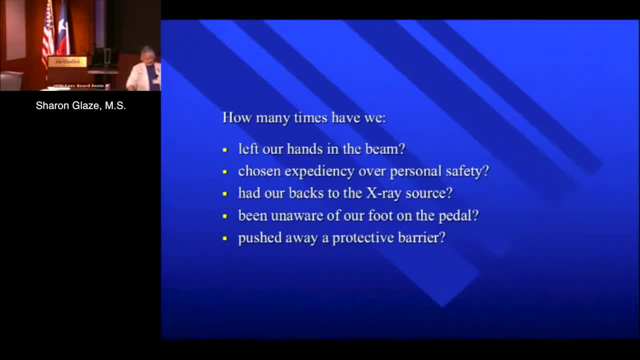 He told me his lead apron wasn't working And so he was doing a research project and he was getting readings on a badge under his apron, And so I didn't have time to go out and fool with this, so I told the tech to put a wrap-around apron on him. 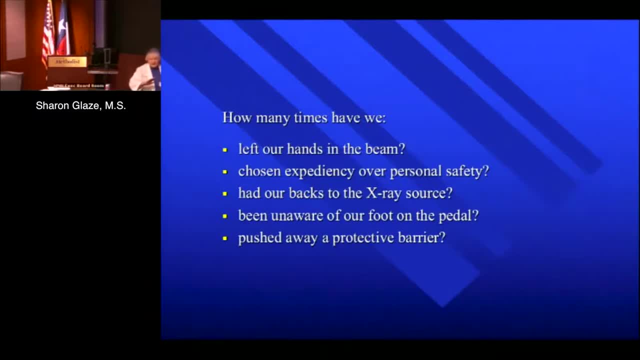 And even though he thought he wasn't turning enough to get the beam hitting him on the side under the apron- and apparently he was Just putting the wrap-around apron on him- got rid of all the exposure under his apron. So with the type work you're doing, I do recommend wrap-around aprons. 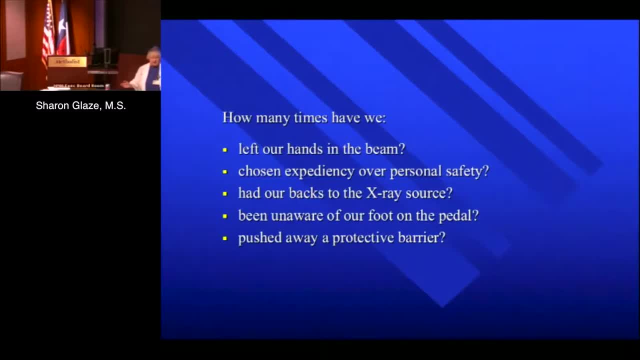 because then you don't have to think about am I turning my side too much or anything, You're just protected. So I do recommend those. Staff protection, Staff protection, Staff protection Protection. yes, Pardon me, How effective is the lead in the first place? 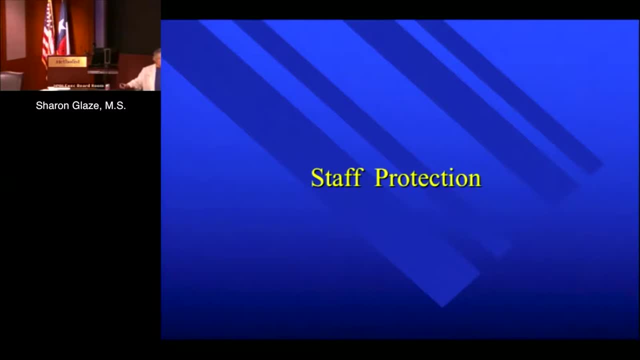 If you were to irradiate directly, does it reflect 99% or 90%? Okay, so, first of all, you're not getting primary beam to that lead. It's made to protect you from scatter, So if I shoot an X-ray beam directly at it, I might get a different number. 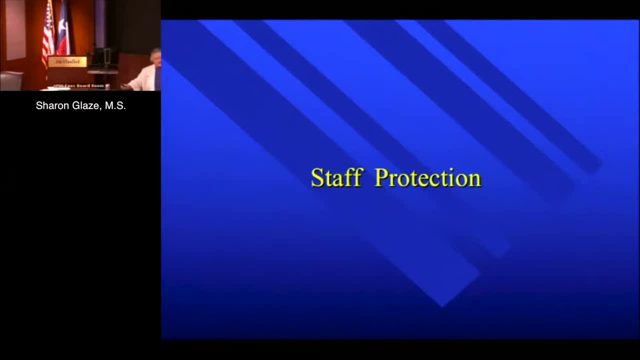 but it actually protects you from about 95% to 98%, So they do a really good job. So, staff protection: it's kind of important, since you're the leader in the room, to pay attention to what you're asking your staff to do. 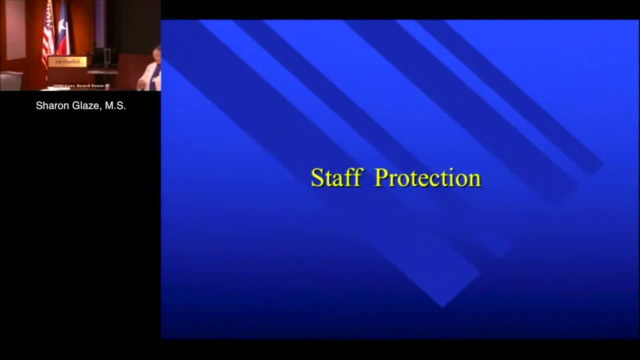 So one example is one time one of the techs said: oh, I have my back to the beam most of the time. So we put a badge on her back and discovered that the way the doctor had her positioned, she was picking up about a rim a month to her back. 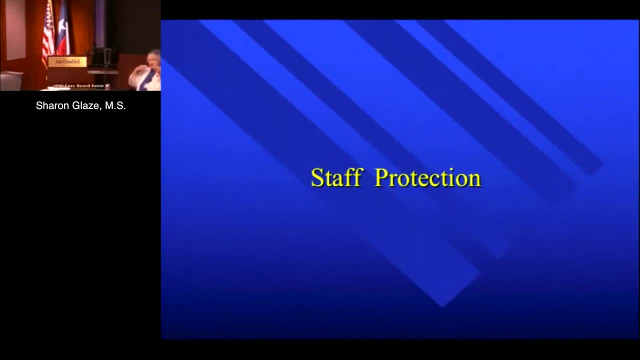 Now she had on a wrap-around apron and a thyroid shield, but still he didn't have her positioned in the right place to adequately protect her. So you need to be aware that someday you're going to be able to protect her. 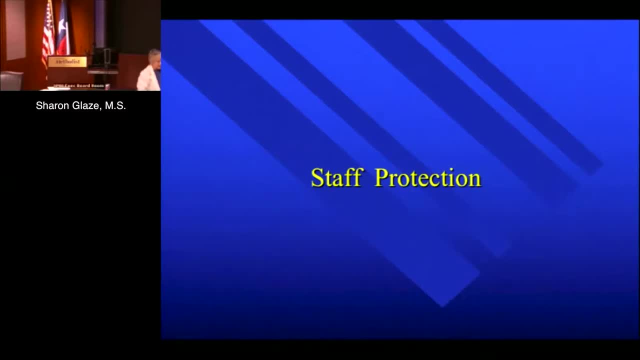 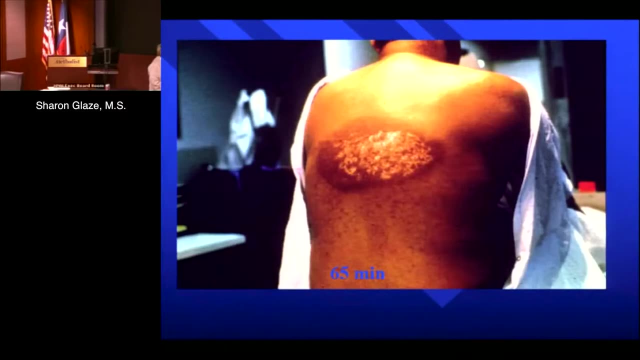 So you need to be responsible for all this staff that's working for you. Patient protection. In the early 90s, about the time stents started being really effective and used, a lot, patients started showing up in the ER with these type of lesions. 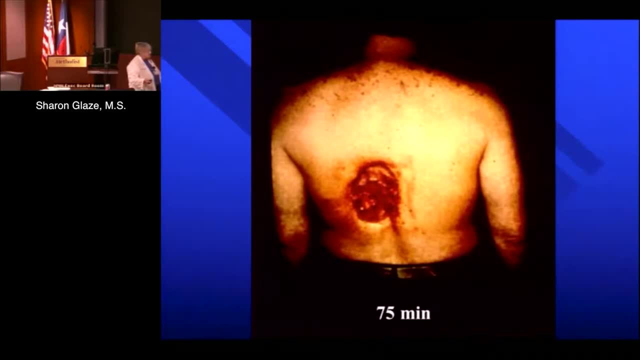 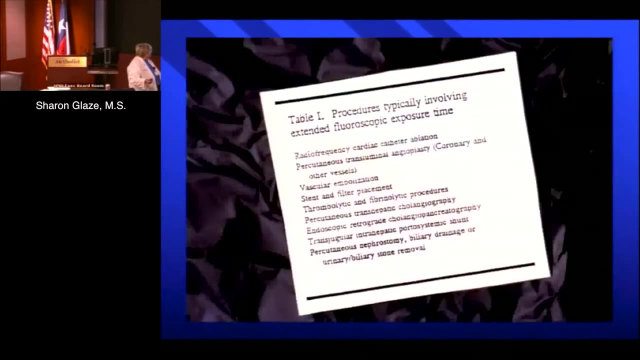 And basically they're all coming out of cath labs And there were all kinds of workshops and basically they determined that these were the type cases that were causing them: angioplasties, actually embolizations, and some TIPs, procedures and other things. 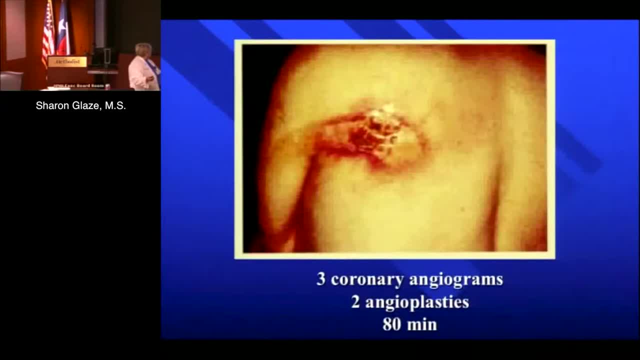 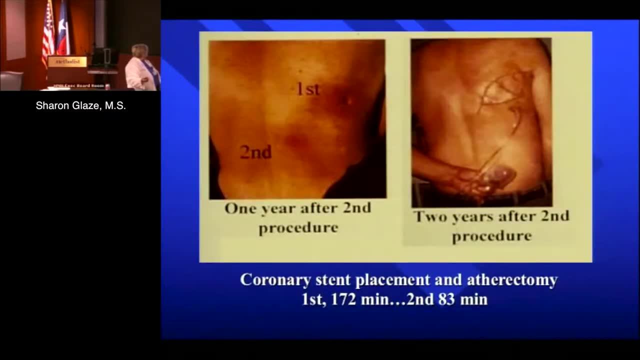 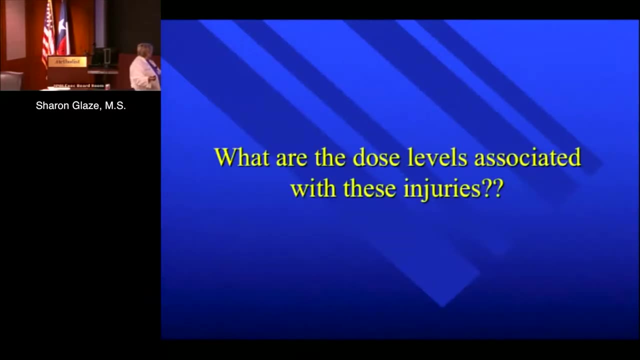 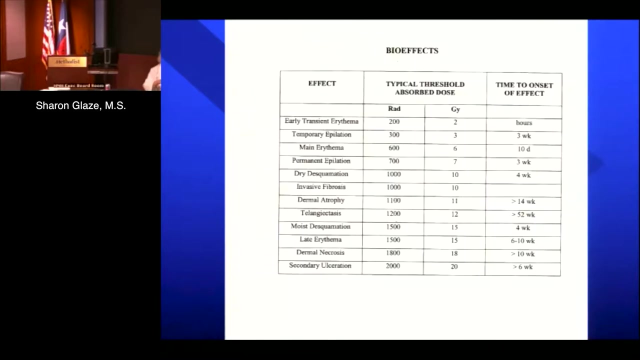 but mostly out of the cath labs. So I have some gory pictures to show you. They required plastic surgery, And what are the dose levels associated with these injuries? Well, I brought that for you to take home with you as sort of a take home, just as a reference. 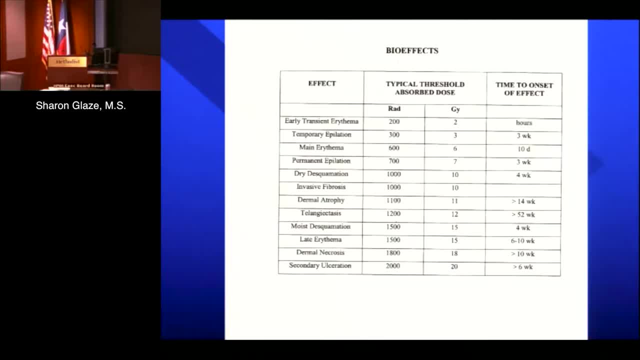 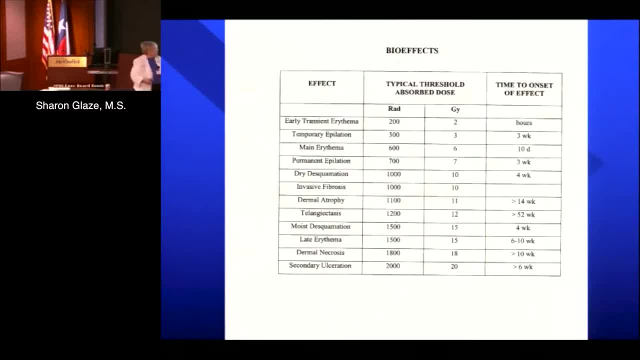 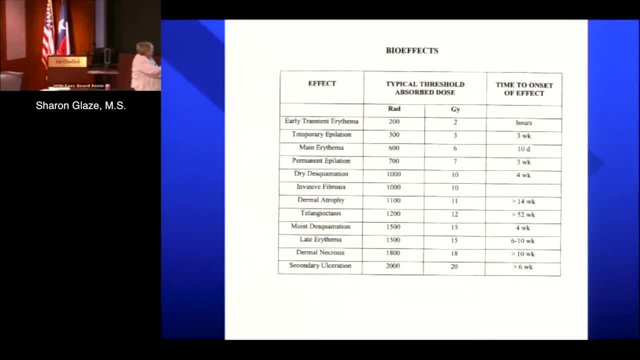 And I wanted you, though, to notice that these don't always show up immediately. Some of them take six weeks, Some take a whole year to show up, So So, as you see your patient from time to time, you could review their back and see how it's looking. 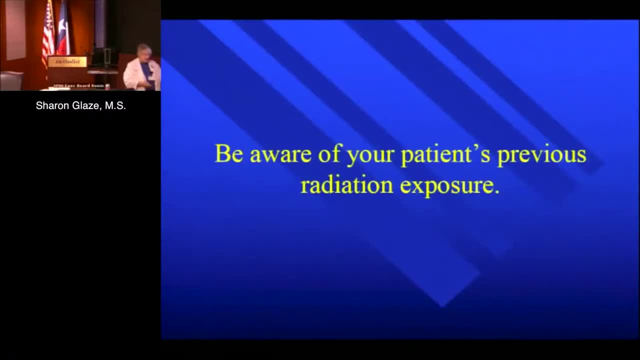 You also have to be sort of aware of your patient's previous radiation exposure. The classic example is they were at Hospital X down the street and had an angioplasty two weeks ago, and now here they are on your table, And so you need to put some thought into that, because that sort of limits your time. 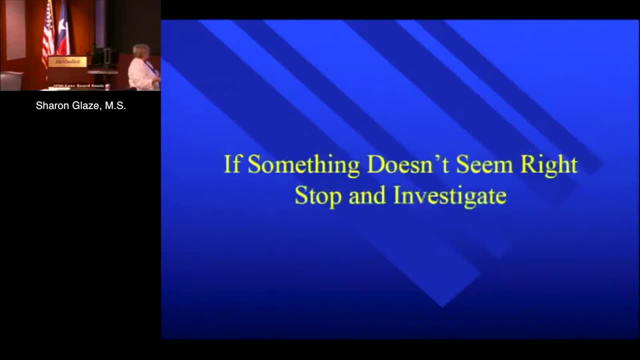 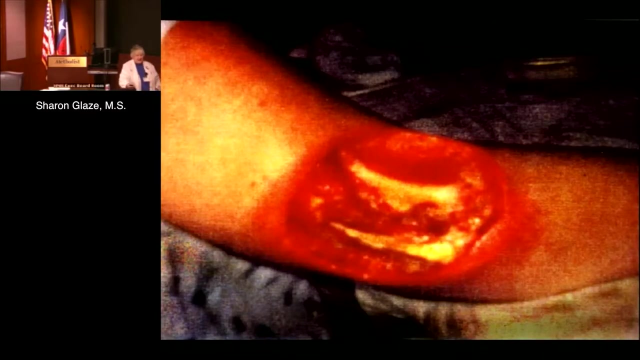 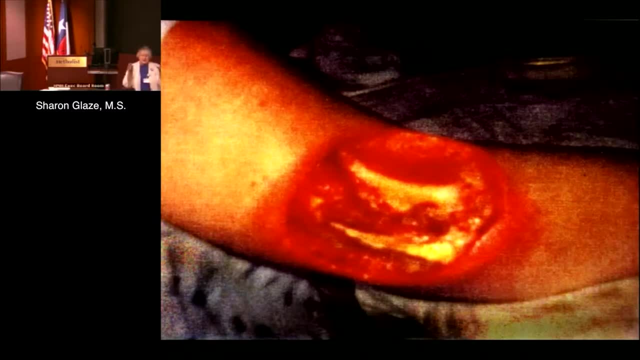 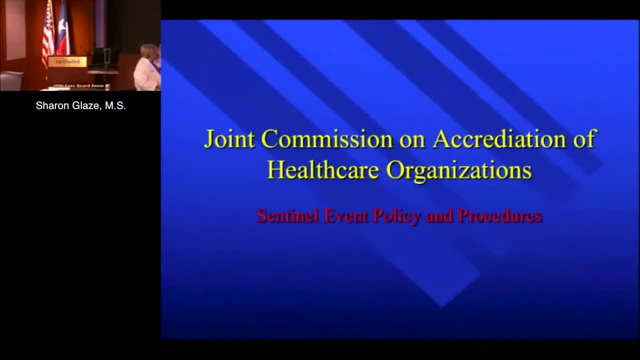 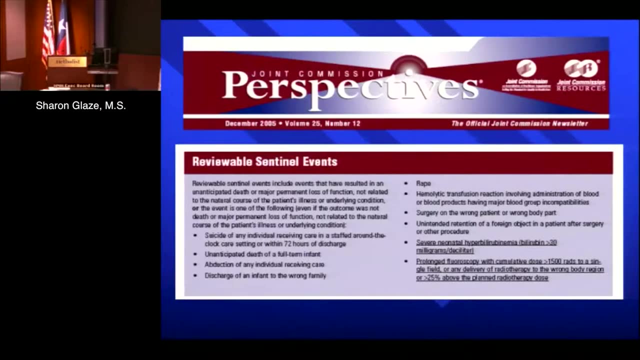 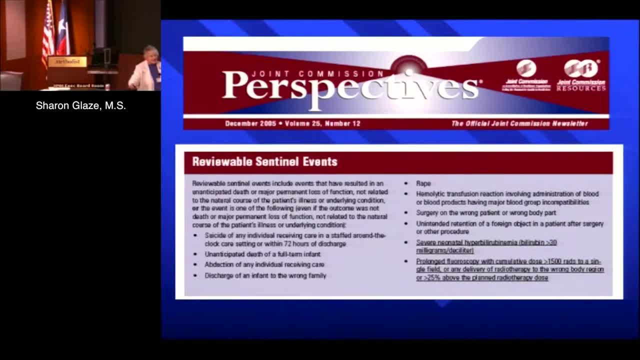 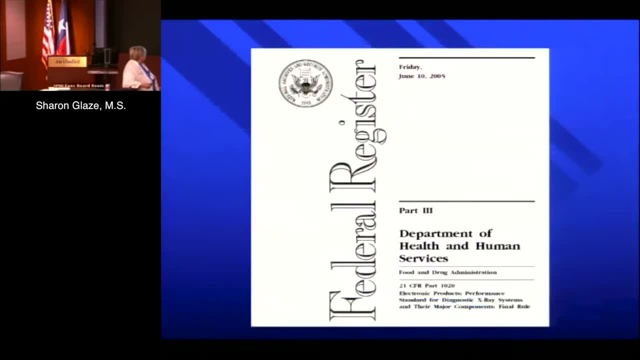 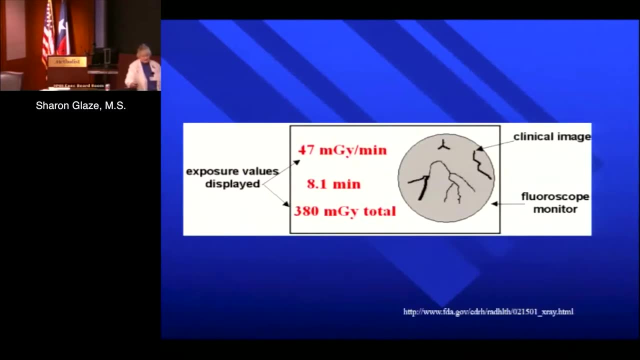 And, And, And, And, And And from the Joint Commission. so we also. I should stop and say that the government decided to do something about this and in 2006 they passed x-ray regs. they do several things. one of them is provide information to you guys as to where you. 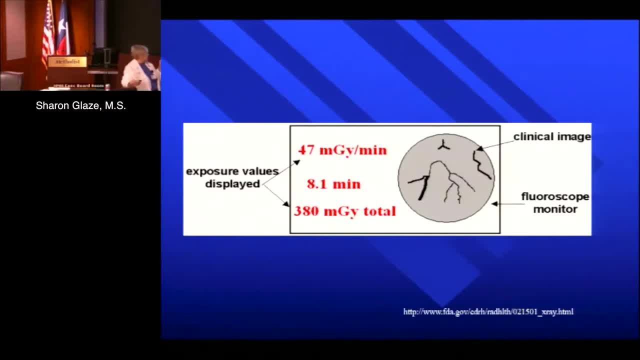 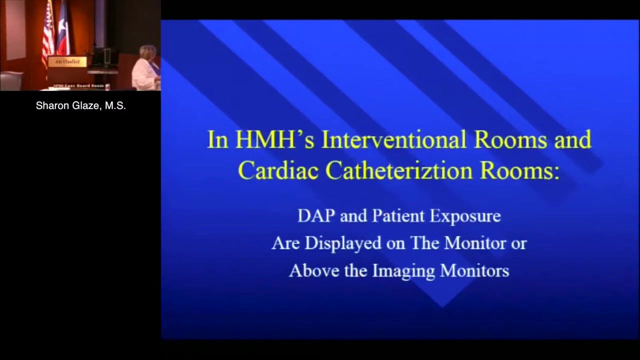 are in the patient's dose situation and what the rate is, and so you know how much time you can know how much flora time you put in and what the cumulative milligray is, and each one of our units has this. they're displayed on the monitor or in cath lab 9. 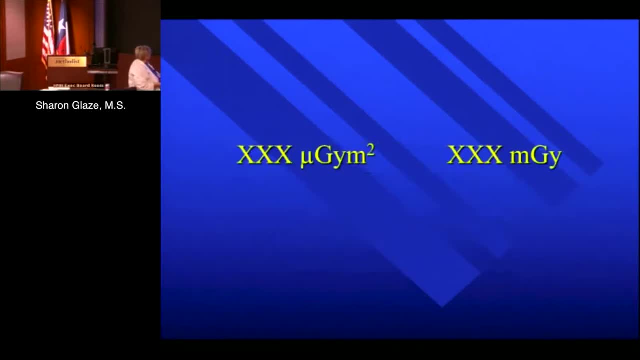 it's above the monitor, and they give you the units in micro gray per meter squared and then also in total milligray. we don't make much use of this because it's it's not very useful information, so this just kind of helps me get my head. 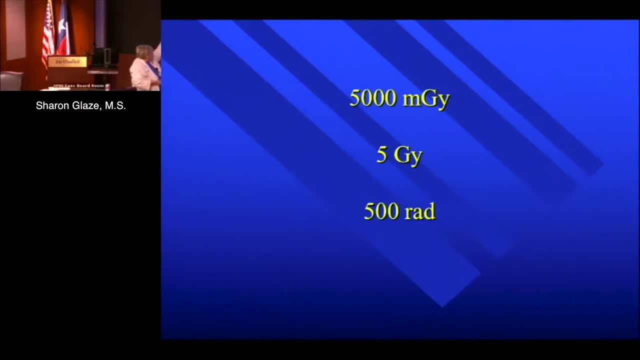 straight, it's like liters, 5000 milligrays, 5 gray, and then, because they're off by a unit of 100, it's 500 grams. why have death meters in the past been so difficult to use? well, the reason is because they read out in dose per area. 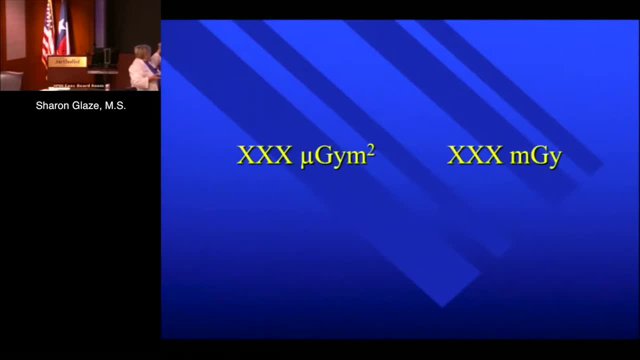 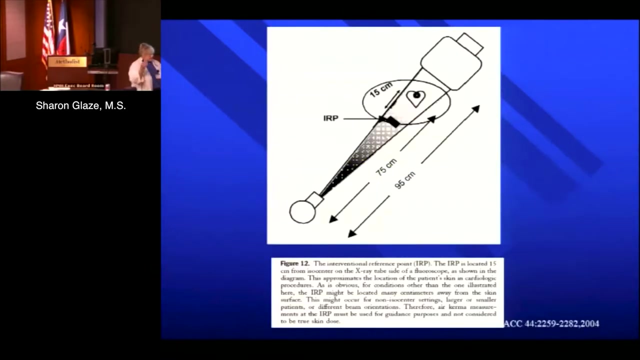 and dose area product, and you have to know the area on the patient's back to give much information out of it. where is the point of patient does calculation for these units? so the way they've decided to do this is they're assuming that this isn't your standard. 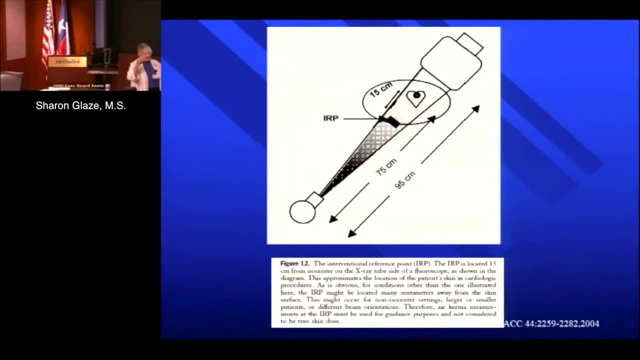 23 cm patient. they're basically saying it's about at 30 cm patient, and so they're calculating back half the distance, 15 cm. so if you put an ISO Center at the point of interest and then measure back 15 centimeters, That's what they're calling the interventional reference point. 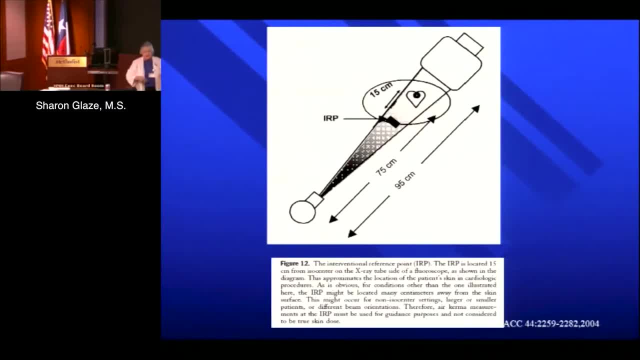 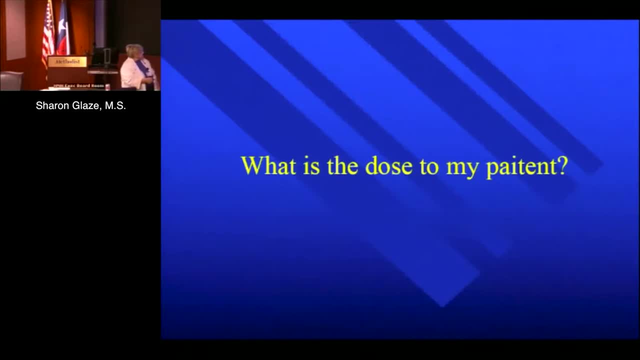 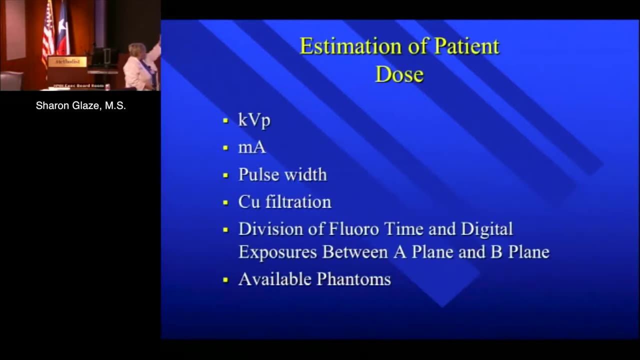 and that's where these DAP meters are displaying the information to. So if you ask me, what is the dose to my patient? Sophisticated new machines vary All of these parameters to give you a great image. They vary: the KV, the MA, the pulse width of the MA. 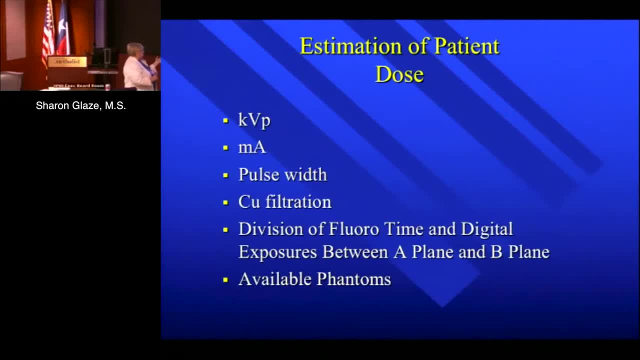 the copper filtration. they pull it in and out as needed And I couldn't guess, to save my life, what your dose rate is. We've taken standard anthropomorphic phantoms in, and the census on your unit prints out how much the technique used. 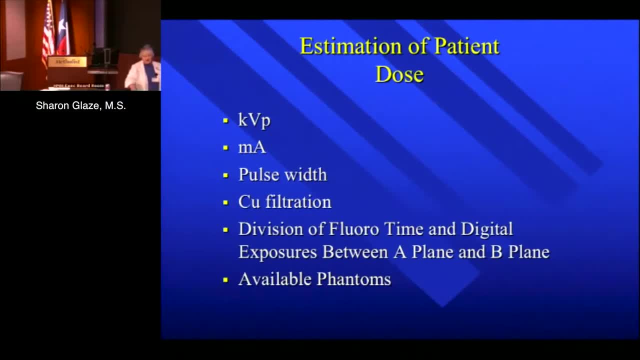 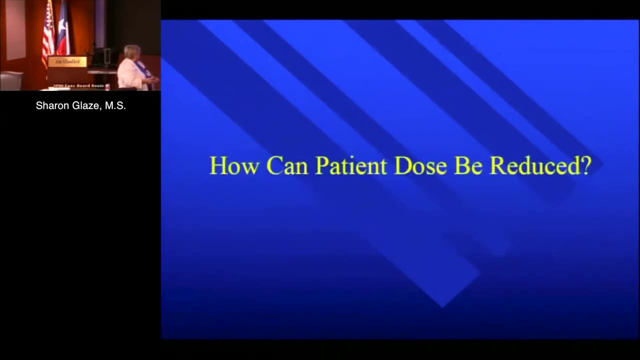 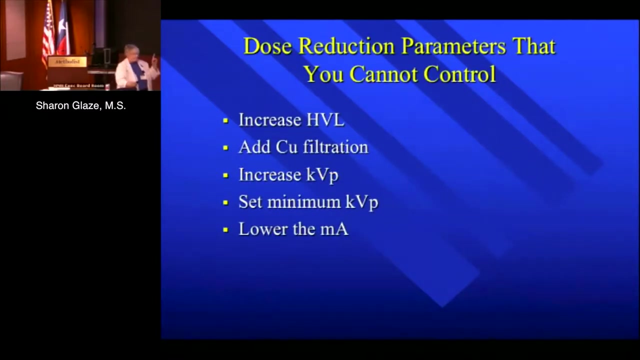 And I can't reproduce it to save my life. So what we're doing is basically using the milligray reading the machine gives us. How can patient dose be reduced? Well, the machines now do it for you. They increase the half value layer, which is basically: 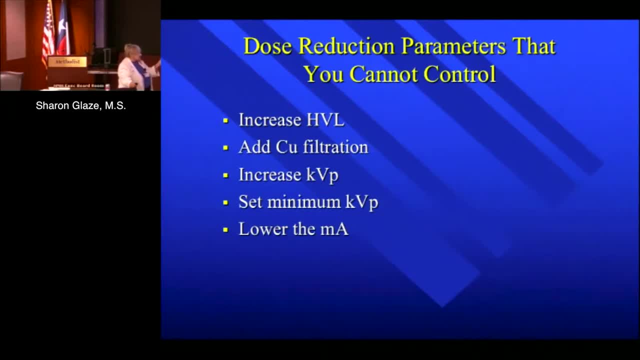 by adding copper filtration to limit the skin dose and use higher energy to penetrate to the image receptor. They use a higher KV because it penetrates better. They set a minimum KV so that it doesn't go too low and just does the skin And they try to lower the MA. 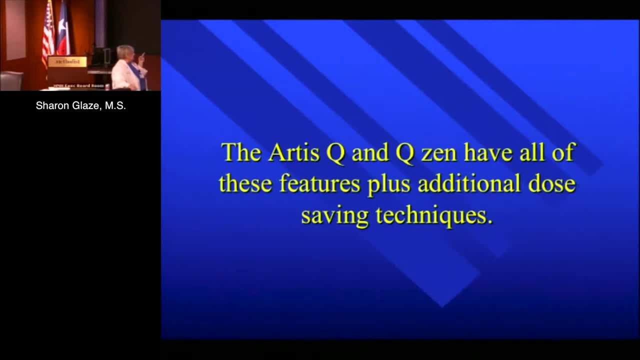 The new machines we have are really have a lot of promise For the future. the artist Q and even more of the QZen have all these features, plus other dose clever, dose savings, things that have been added to these units, And I think they're going to have a very, very bright future here at Methodist. 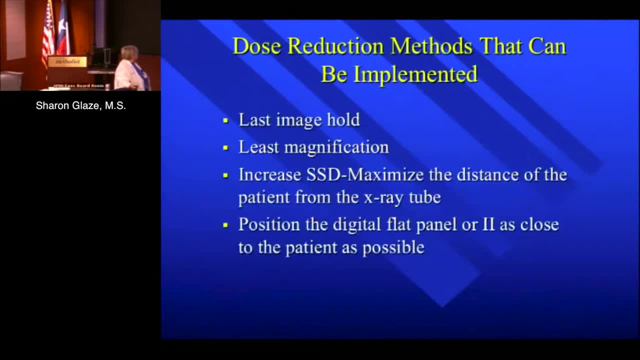 helping us keep patient doses low and your dose lower. It's important to use as little magnification as you can, because the dose goes up with the magnification, And it's important to keep the black panel as close to the patient as you can without ruining your sterile field. 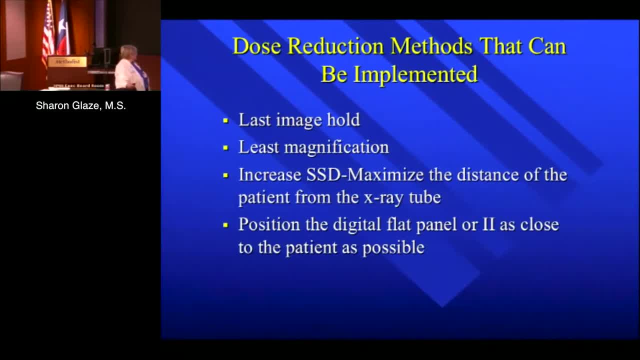 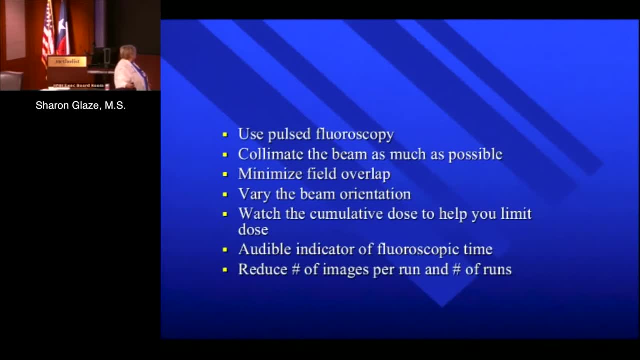 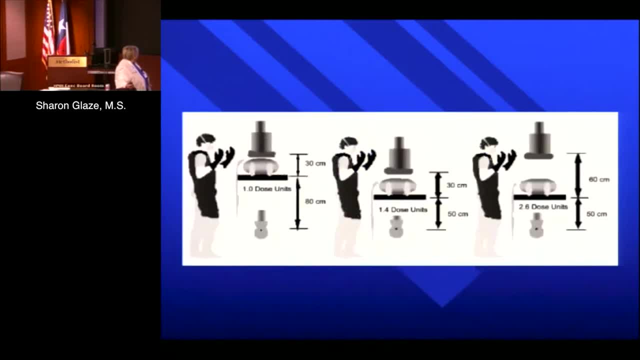 It's automatically selected And it's important to keep. just like inverse square law helps you, It hurts the patient if you accidentally like here it's one dose unit because the patient's far away from the X-ray tube. Here's more like your situation and it's more. 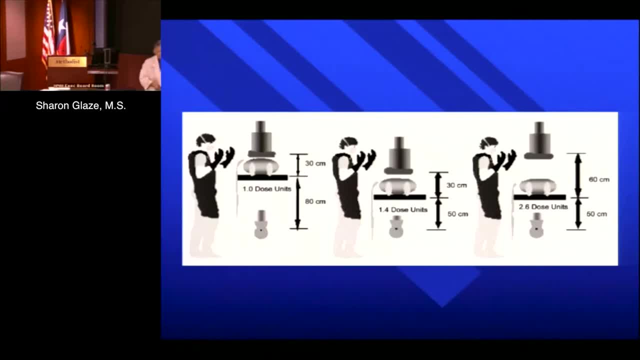 but it's still acceptable if you get them too close to the X-ray tube. Now I don't worry Much about this in the cath labs because in order to angle the tube you have to have it sort of mediated. I worry about it with C arms and surgery because they don't swing them so much. 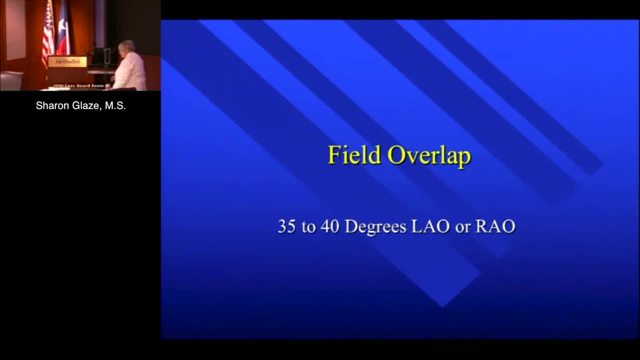 Okay, One talk about field over lab. So part of the problem is you go LAO and you go RAO and you're hoping that this is what's happening on the lab And you're hoping that this is what's happening on the patient's back. 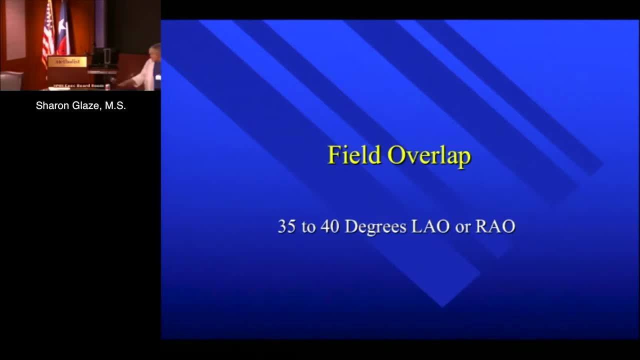 That the fields are totally separated, But in reality that's not the case. It's more like this, And you can kind of see that they're overlapped, And this is because the tech comes through and recenters up the center of the field. 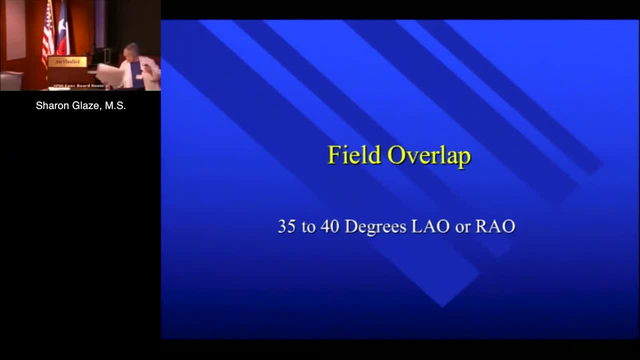 to let you see what's going on more appropriately, And we're almost through Pulse. fluoro requires careful inspection because you would think, if you're running continuous and it were four hour per minute, if you cut it and have it, you'd go down to two, and then down to one, and so forth. 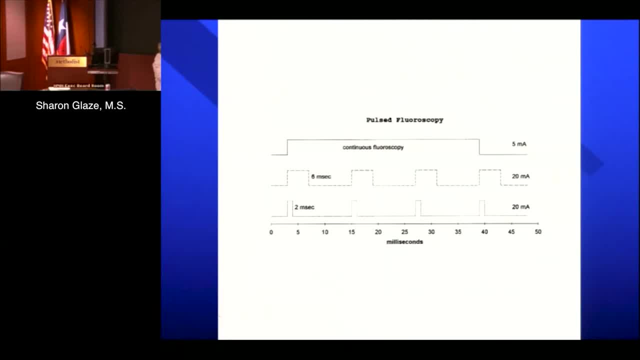 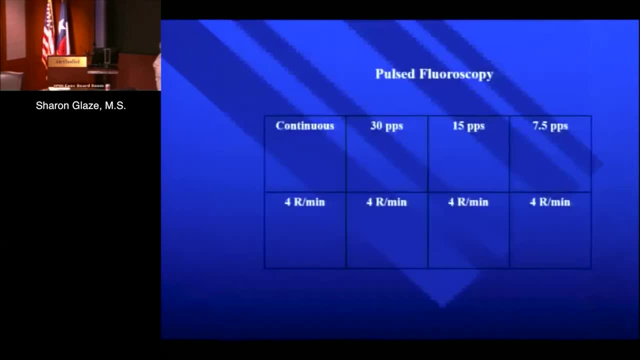 But in the beginning they can actually alter the pulse widths to give you better image quality. And so in the beginning of pulse fluoroscopy I had to do a lot of work. I had the experience of going in and it was all the same. 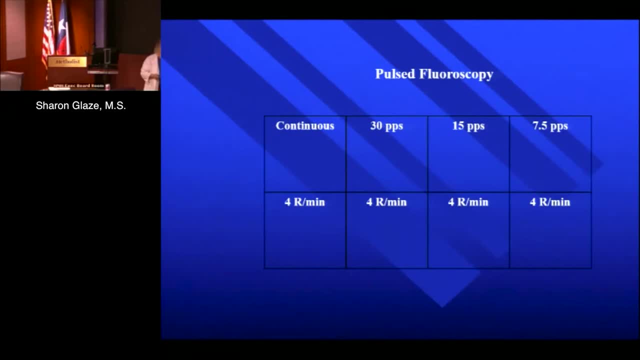 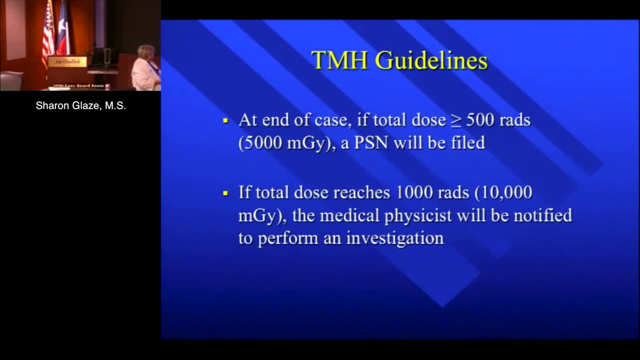 no matter how much they were pulsing it, because they had widened the pulse width. So this doesn't tend to happen anymore. Okay, As far as dose goes, Houston Methodist has some guidelines And at the end of the case, if the total dose is greater than 500 rads. 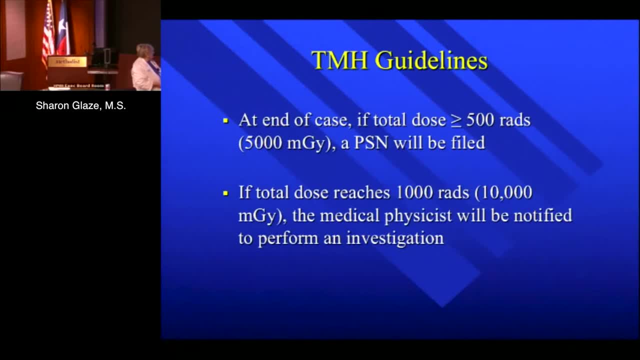 or 5,000 milligray of PSN is filed and if it reaches 1,000 rads or 10,000 milligray, then I have to go or one of my associates goes and we will try to decide if this was high enough to be 1,500 and could it be a simple review. 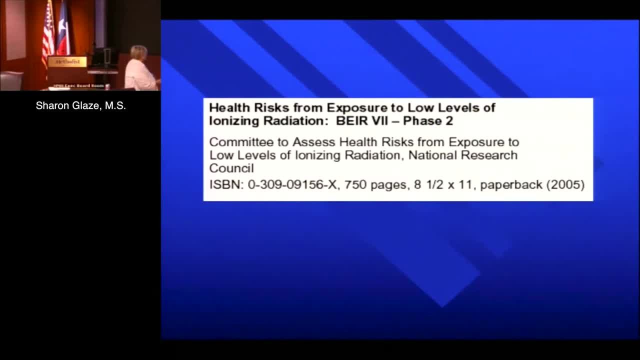 Okay, I'm going to read you two or three little things and then we're done. So the only irradiated population is still Hiroshima and Nagasaki from World War II. There's some cases of like early radiologists, but the only whole body irradiated group are these people. 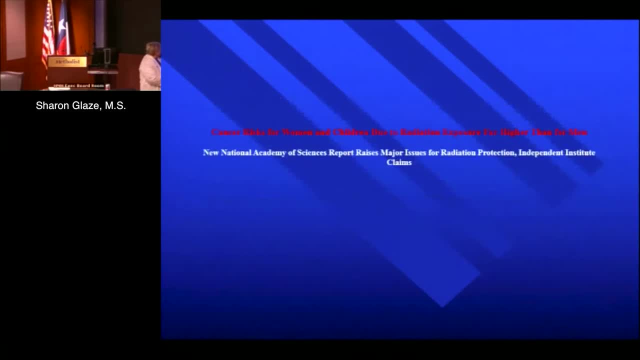 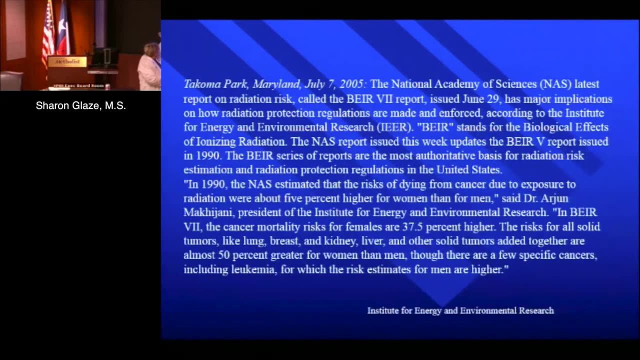 and they reassess their information all the time. Okay, And the report is actually the Beers 7 report, I believe. Let me see The Beers 7 report And so I want to read this to you. In Beers 7, the cancer mortality risks for females are 37.5% higher. The risks for all solid tumors like lung, breast, kidney and liver and other solid tumors added together, almost 50% greater for women than men, though there are a few specific cancers, like leukemia, which were higher for men after exposure to radiation. And then we're always concerned if you go into pediatric cardiology. 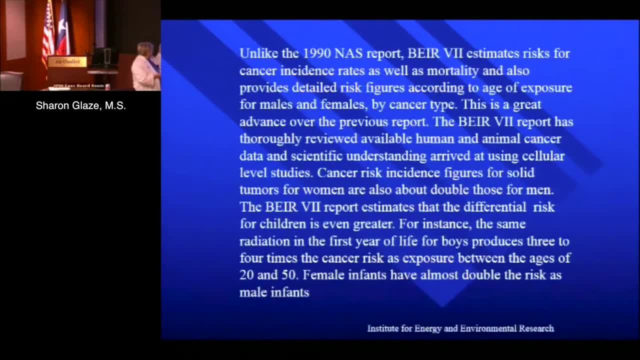 because Beers 7 estimates the differential risk for children is even greater. For instance, the same radiation- Oh Okay- in the first year of life for boys produces three to four times the cancer risk if exposure between ages 20 to 50.. 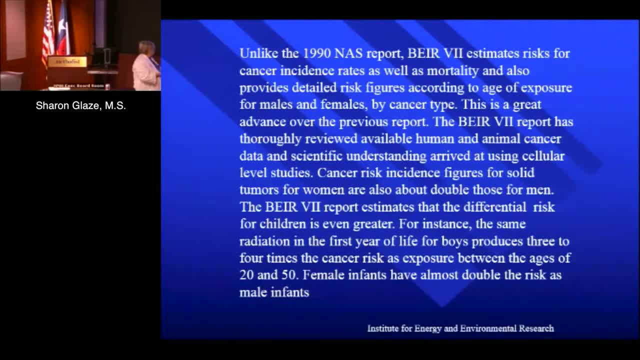 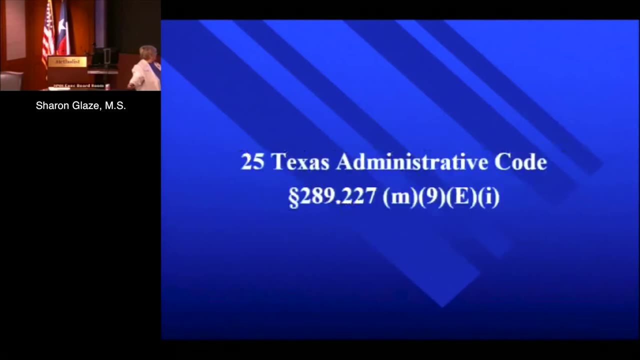 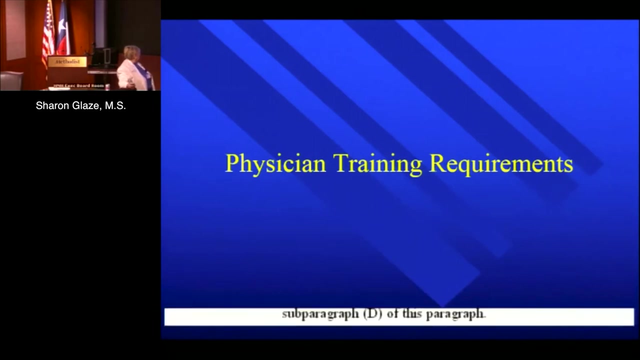 Female infants have double the risk as male infants And I don't know if that's because of breast cancer or what. the cause of that is OK. the last thing is Texas passed a law which was going to require physician training requirements, And actually they were requiring. 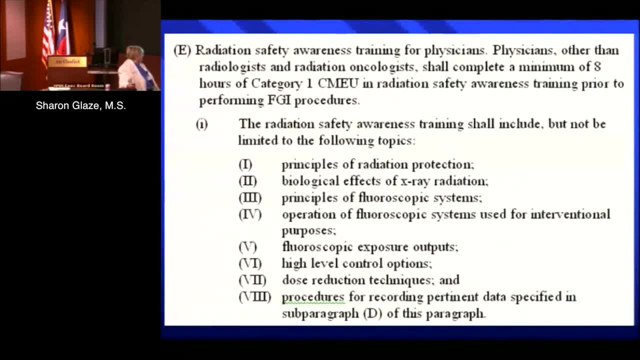 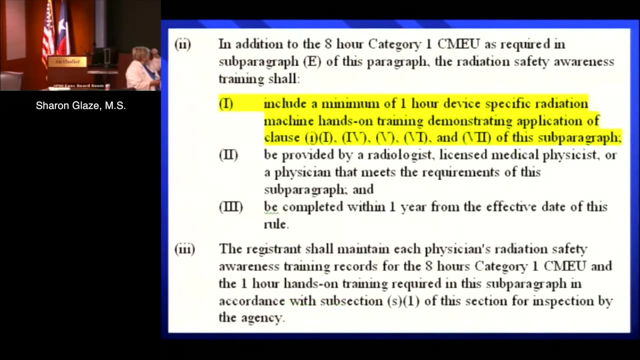 a minimum of eight hours of training in x-ray equipment And I always thought that was a little excessive about one hour of this And maybe some radiology would be about all you guys need to know to protect yourselves and your patients. But actually, and then it included. 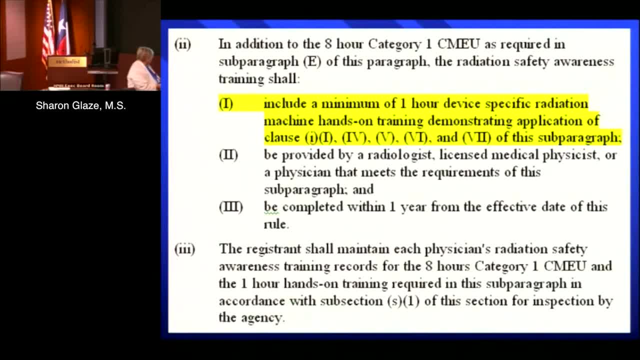 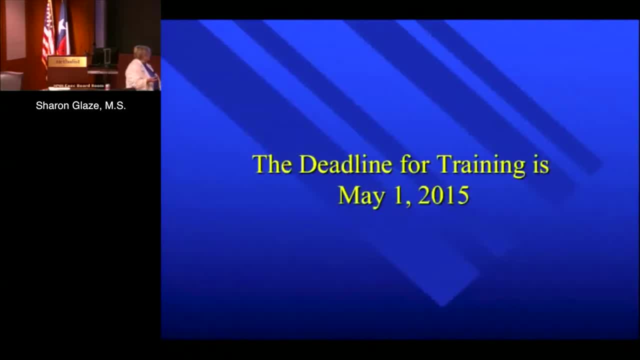 one hour extra of unit-specific information. But actually the Texas Medical Association lobby was very effective because they postponed it indefinitely, And so for people like me, we really think everybody needs a little training, maybe not being tortured with eight hours, But people need a little training of what to do. 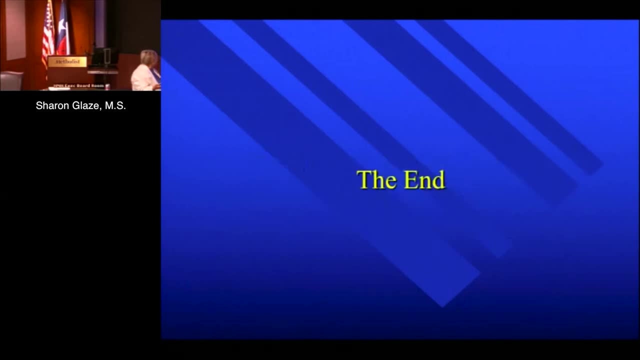 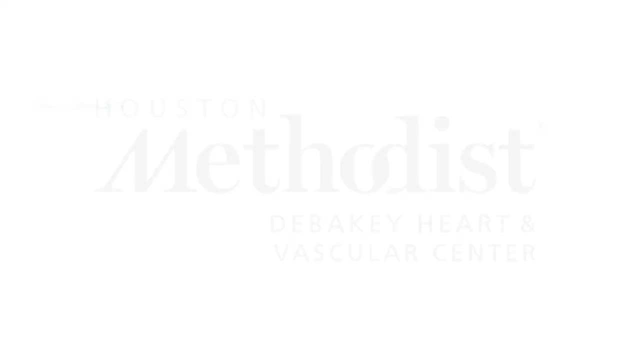 And now they've totally negated it, And that's all I have, Thank you, Thank you.